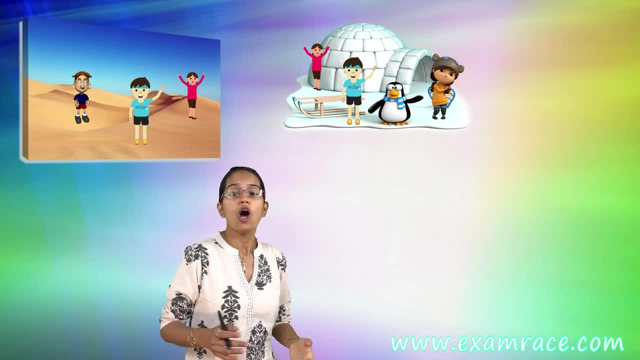 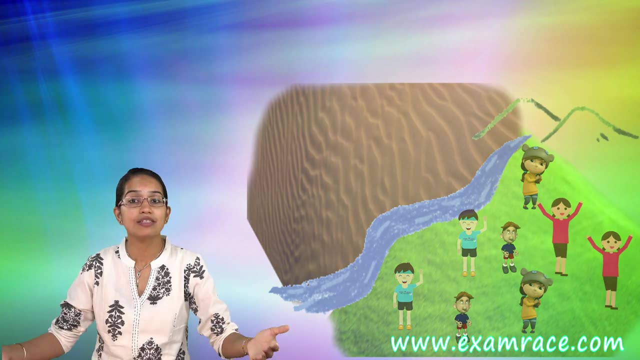 very few population or people residing in those areas. On the other hand, regions close to the riverbeds have numerous population that could be seen and that's because of ample of water availability. a lot of agriculture that could be seen and a lot of agriculture that could be seen. 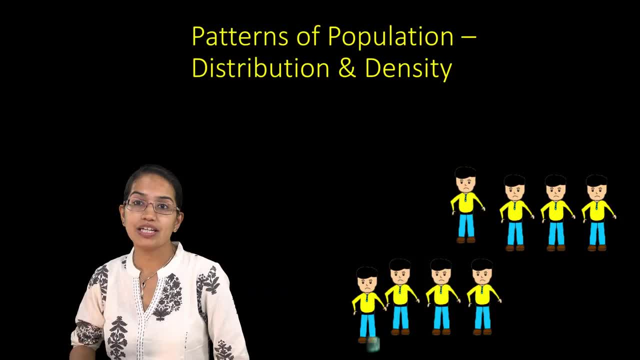 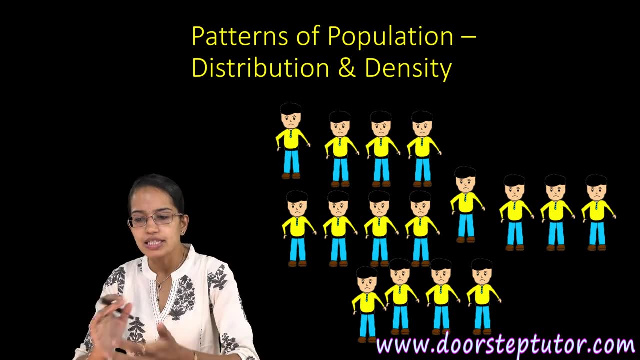 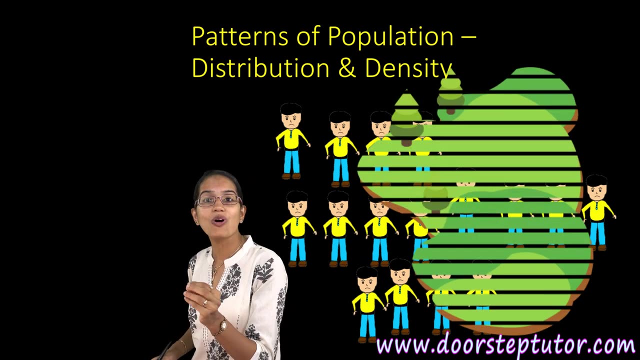 Again, population growth is very, very interesting. So, as you see, you have a constant increase in the population. that is seen. This increase in the population governs a very interesting fact: that 90% of the population lives on only 10% of the area. So understand the fact that that 10%. 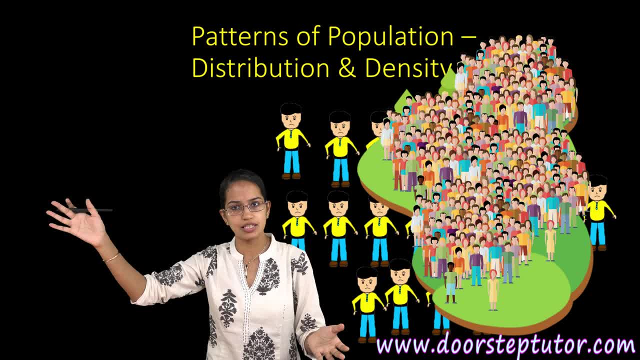 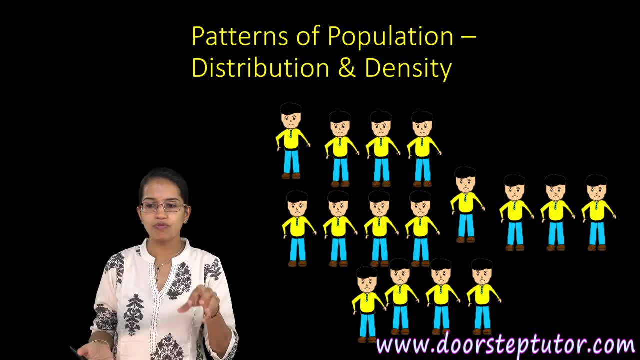 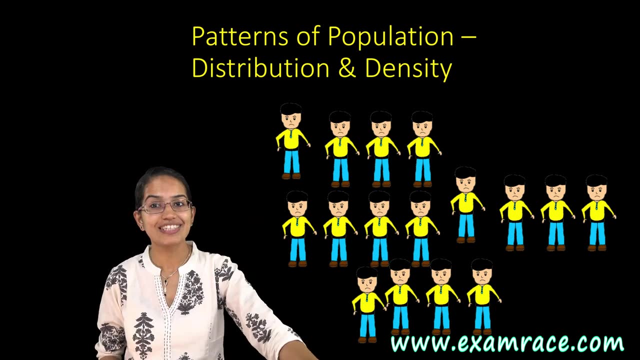 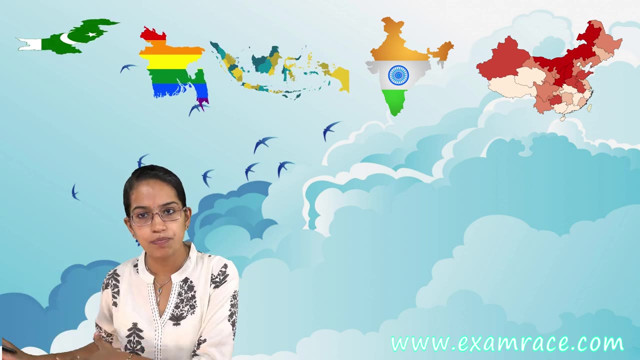 has to have that much resources so as to sustain the 90% of the population Again in the world. if you succeed, you have 60% of the population which resides only in the 10 most populous nations. Of that 10's most populous nations, 6 are in Asia. that's mainly China, India, Indonesia, Bangladesh and Pakistan. 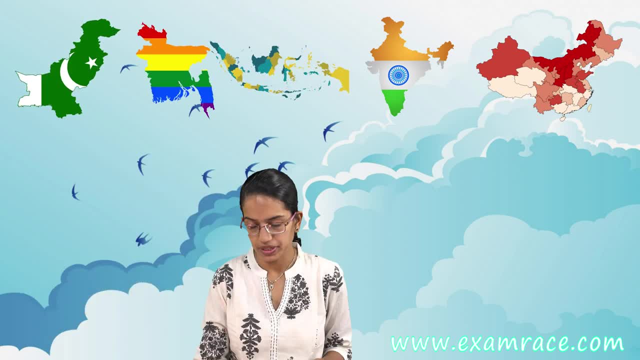 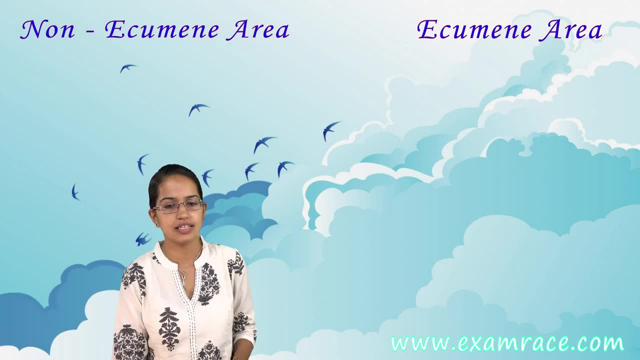 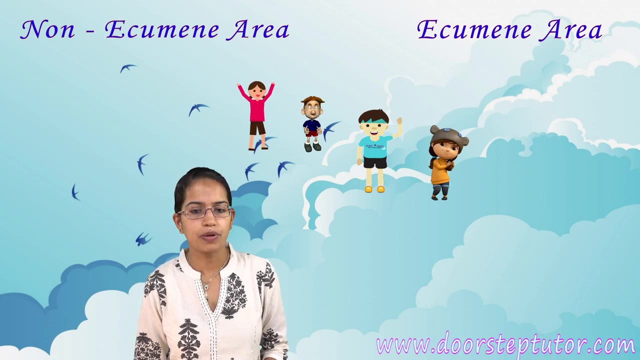 so these are the place where you have the most populous nations, The areas where you have a lot of population, known as the ecumen areas. non-ecumen areas are the regions where you have less population: ecumen and non ecumen as the two population areas that are seen the next. 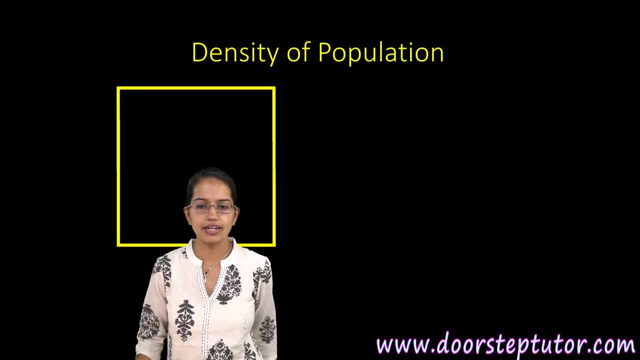 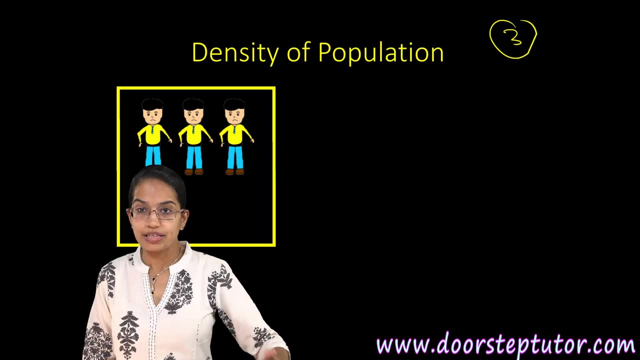 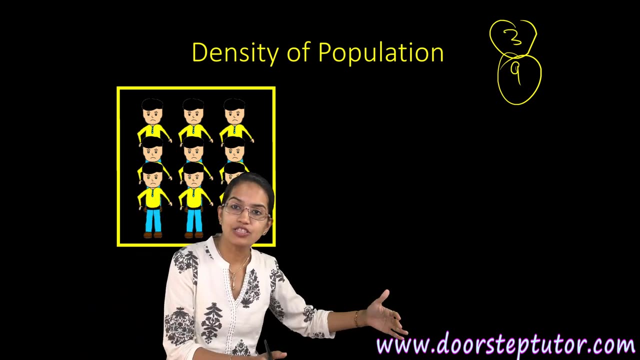 is population density. now, let's say this is a piece of land that we have here. on this piece of land, you have three persons that are living now. with population rise, you have few, more and few more. now you have nine people on the same patch of land. so the same patch of land which was able to sustain three. 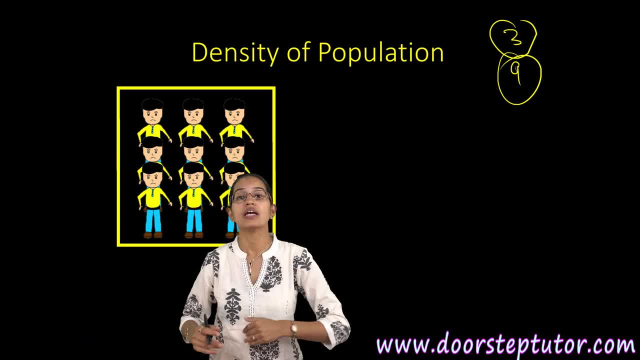 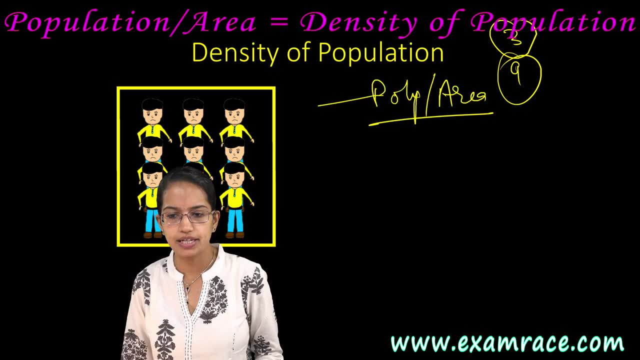 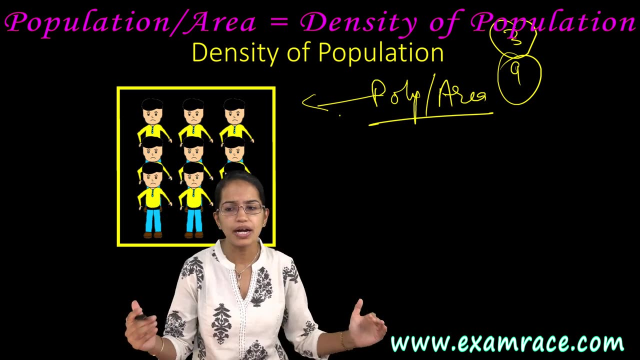 people earlier now has to sustain nine people, and that's what is the population density. the population per unit area that could be explained is the population density, and it's dependent on the size of the land that is present on the parcel of the land. some of the most densely populated areas of the world are 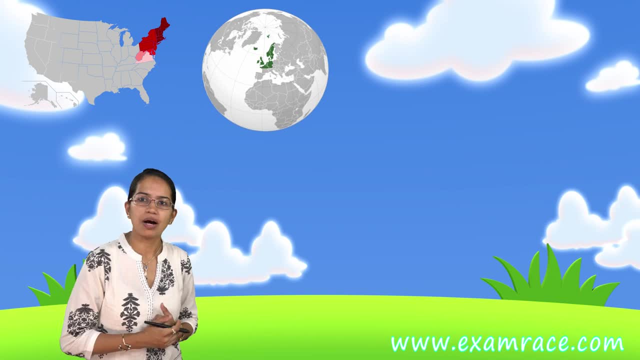 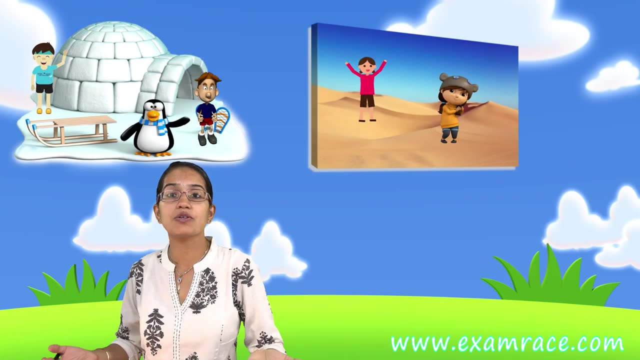 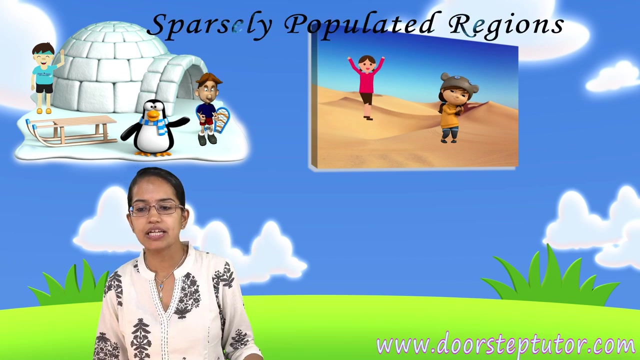 northeast parts of America, northwestern parts of Europe, Southeast Asia and Eastern Asia. besides that, the polar areas, the desert areas, are the areas where you don't have even one person per square kilometer, so it's very sparsely populated. so sparsely word means very few, so there is very less population. that is seen. the next is what? 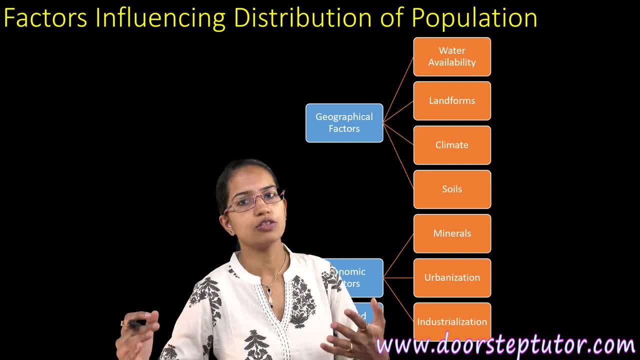 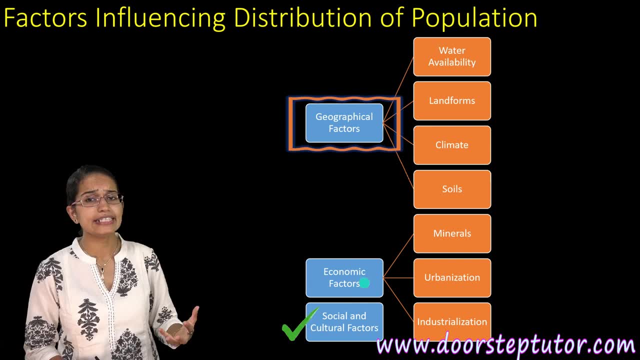 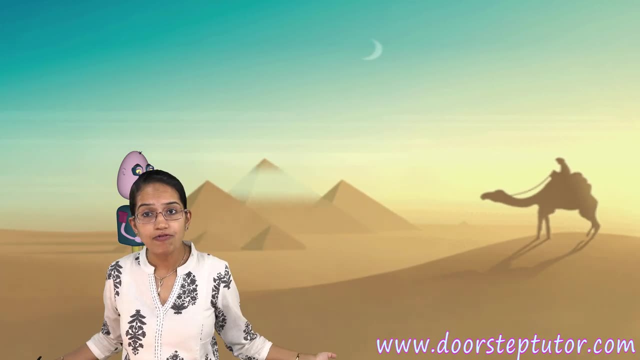 are the factors that affect the population. so, indeed, we classify those under three major factors: geographic factors, economic factors and social cultural factors. when I say geographic factors, the first is water availability. if I go on to a desert area, definitely it would be hard for people to live, but on the other hand, 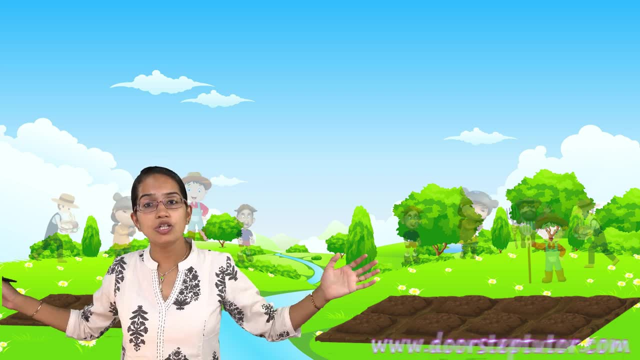 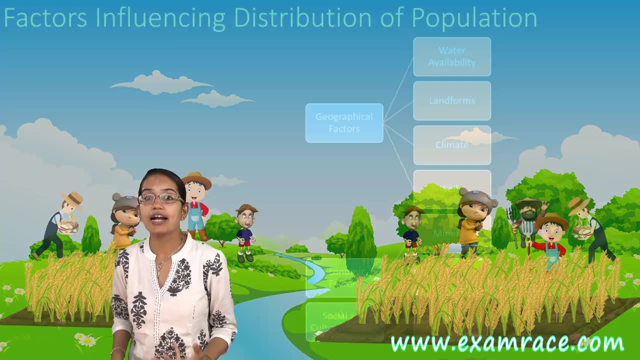 if I go to Indo Ganga plains, you have a lot of population that would be residing there because ample of water, ample of agriculture, happy life, on the other hand, landform. so if I go to Kalash Mansarovar and say there is a huge residency set up, 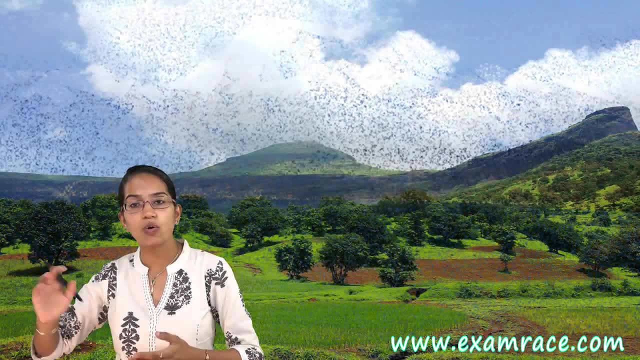 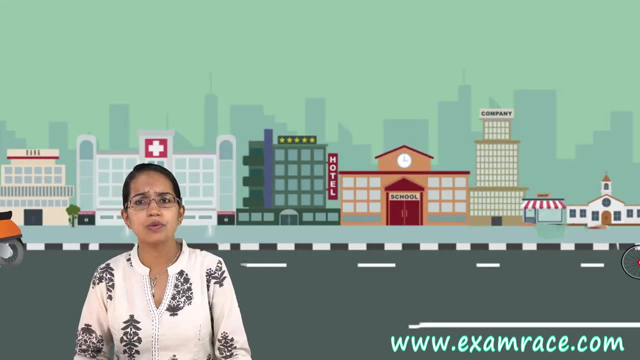 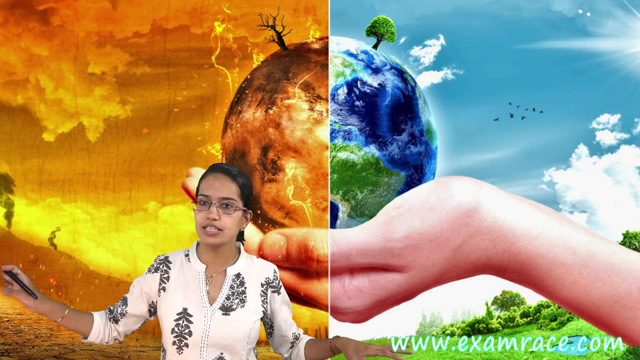 here, of course there is not, but again, in a Ganga Duaab area, I would find a lot of people that are residing, the reason being the landform, the accessibility, the better transport facilities that could be available based on the landform. the next is climate. so extreme climate speed, extreme cold, extreme hot. it's not good. 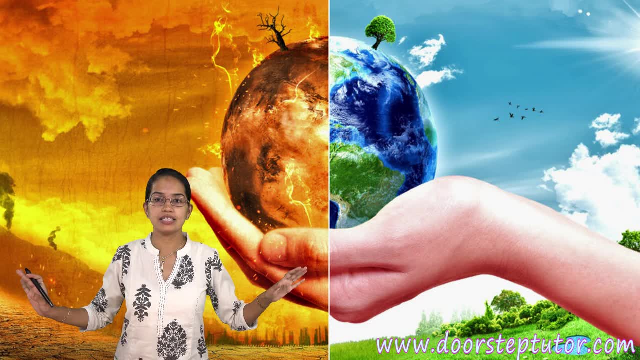 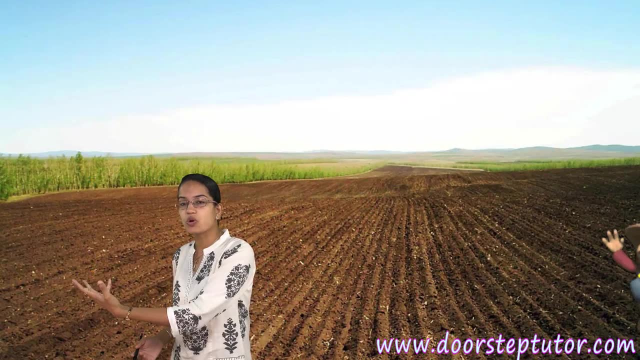 for human conditions. on the other hand, pleasant weather conditions like Mediterranean would be a region where you would have ample of population. that could be seen soil, so a fertile soil would be home to lot of agriculture. you can have lot of intensive agriculture, lot of farming that could be present. 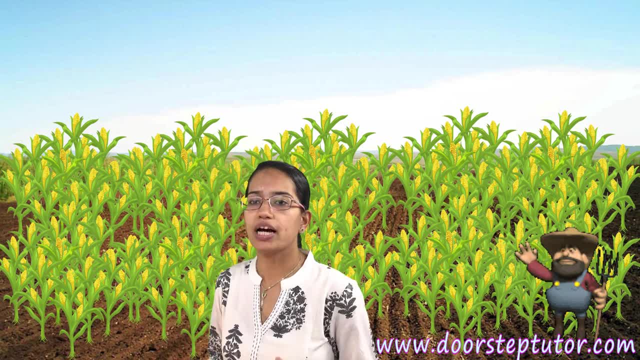 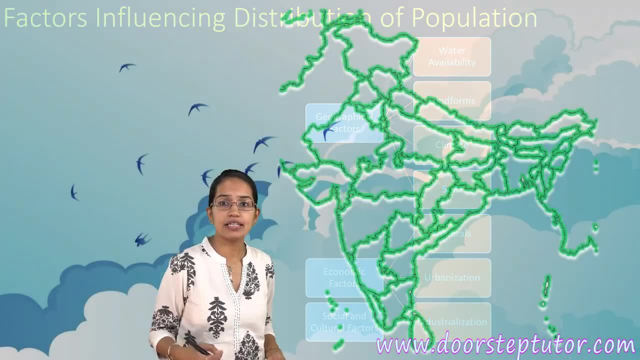 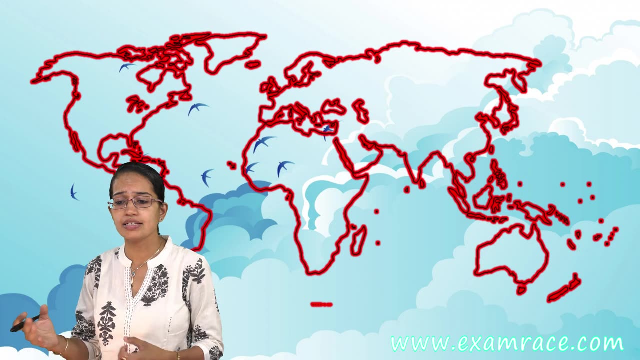 here. so loamy soil, fertile soil, clayey soil are the areas where you would have agriculture and, as a result, more population, economic factors. definitely minerals. in india, we say across the globe we say regions of the cove areas in japan, where you have a lot of. 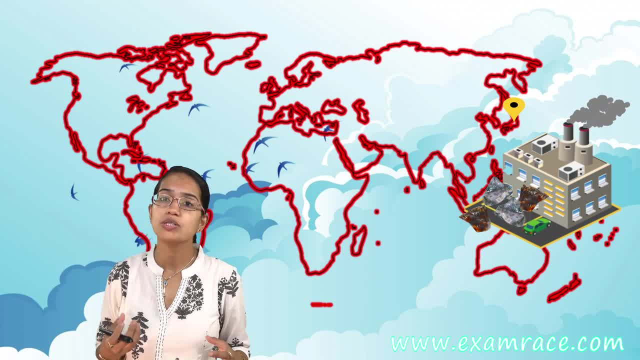 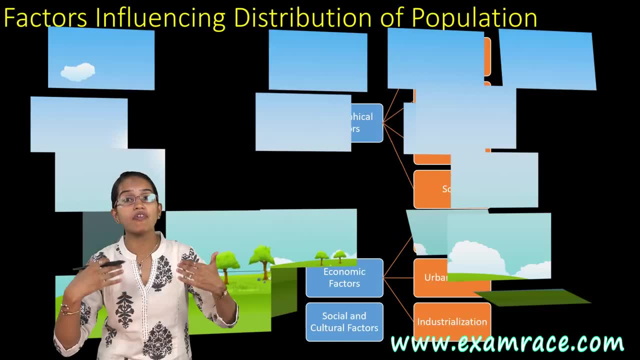 industries as well as lot of minerals that are seen. so cove osaka area is one of the major industrialized areas, highly populated regions of japan. that is seen similarly. in wake of urbanization, we have a lot of labor that's coming in from the rural areas to the urban areas. 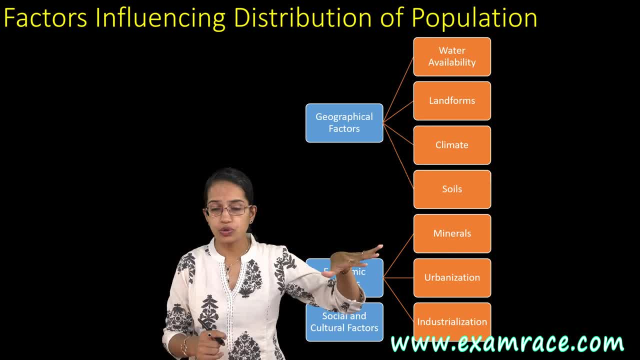 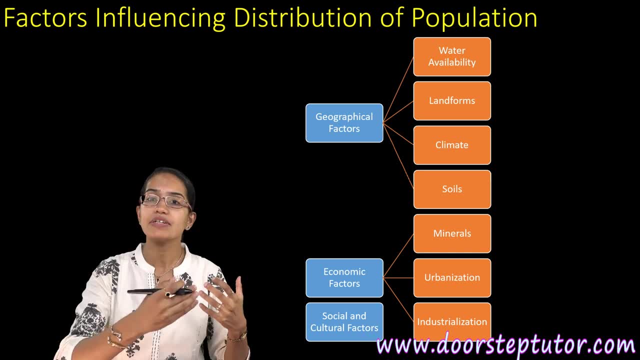 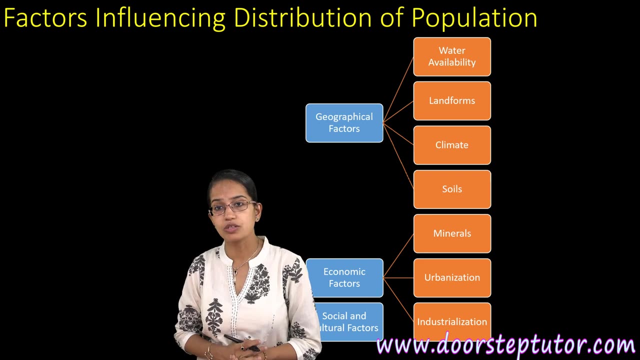 the philadelphia, boston, mexico, new york- sorry, new york is the area where you have a lot of population that is being accumulated and we say this is a kind of megalopolis that has been developed in the vicinities of new york till boston. you could say so. that's how you have the. 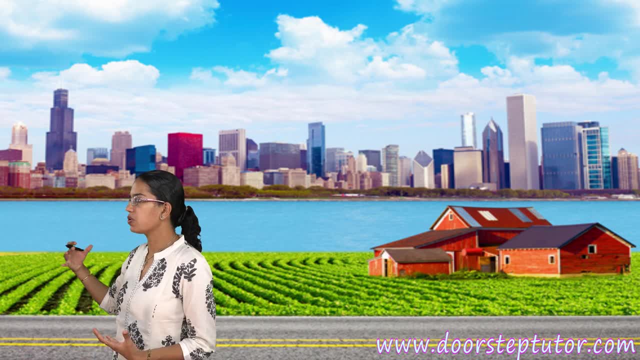 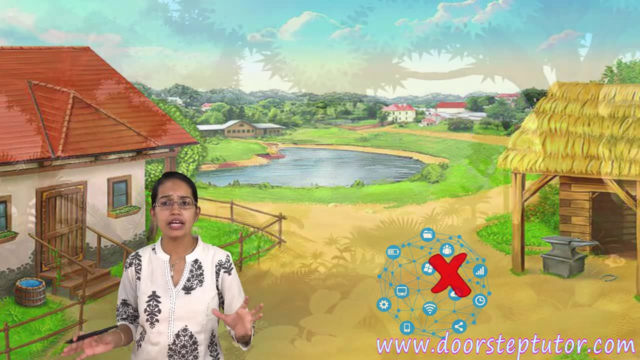 wake of urbanization. however, on the other hand, you have areas of urbanization that are seen as a lot of labor that is coming in from the rural areas where you don't have a good connectivity, good urban area, a lot of rural area, the rainforest areas of amazon basin, congo area won't be the areas where you would have a lot of population. 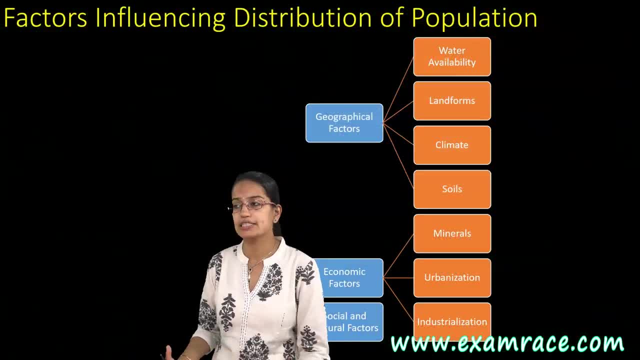 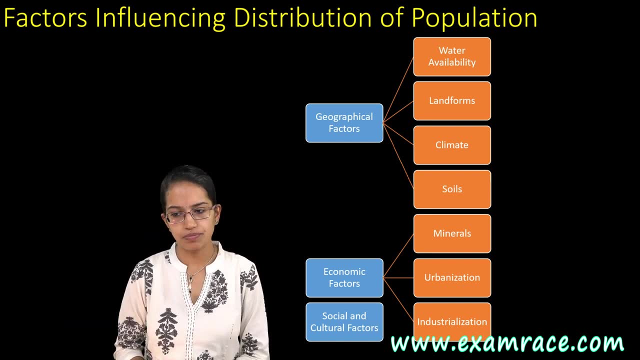 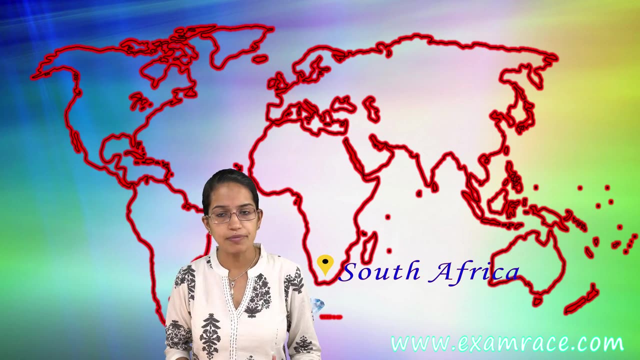 that would be seen. so social and cultural areas factors are another important factors that lead to binding a stronger, the binding more the population that would be inhabiting that region. similarly, in africa also, you have the south africa regions where you have the diamond mining, gold mining that's seen. you have the zambia copper mining belt that is seen in katanga. so those are. 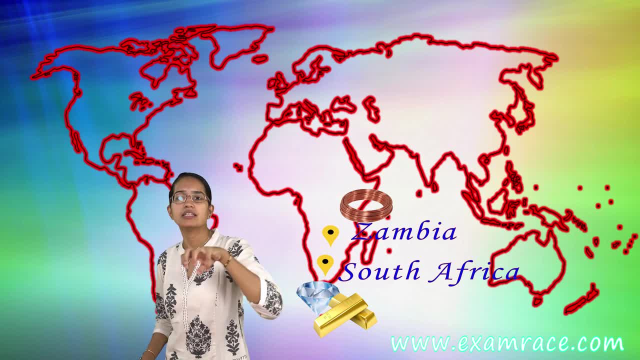 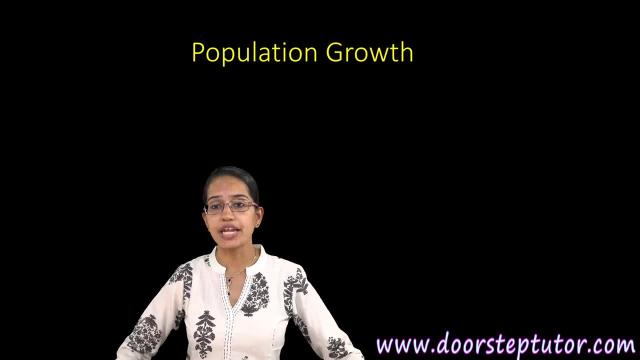 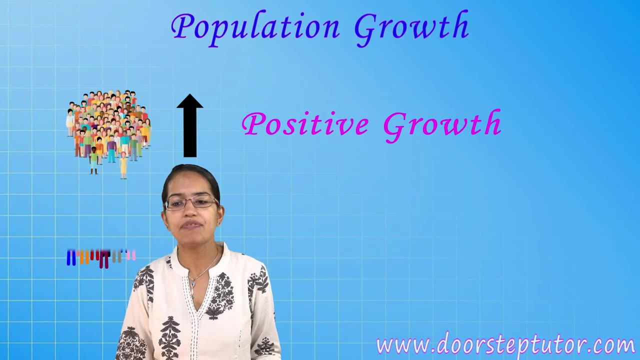 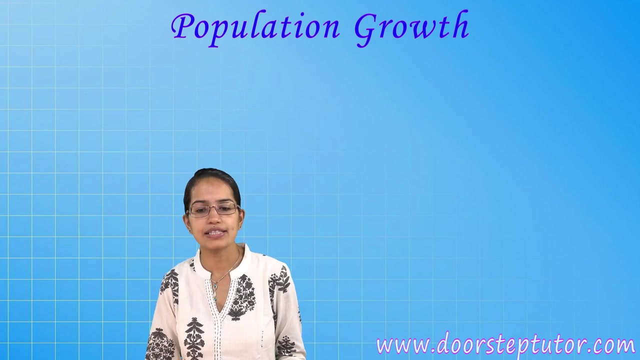 some of the areas where you have population uh presence or highly populated areas, those are present population growth, a very, very important term now, population growth: if it is increasing, i say population growth is positive. if it is declining, i say it is negative. Now this population growth could be classified as natural population or 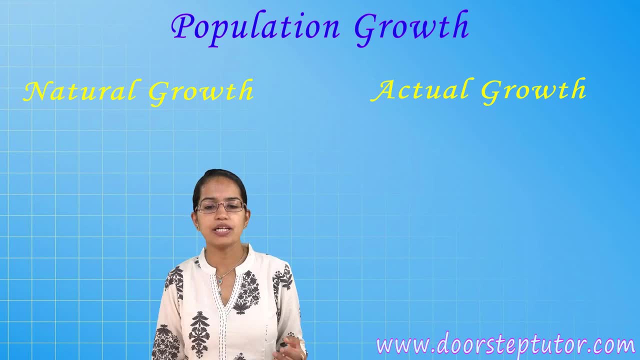 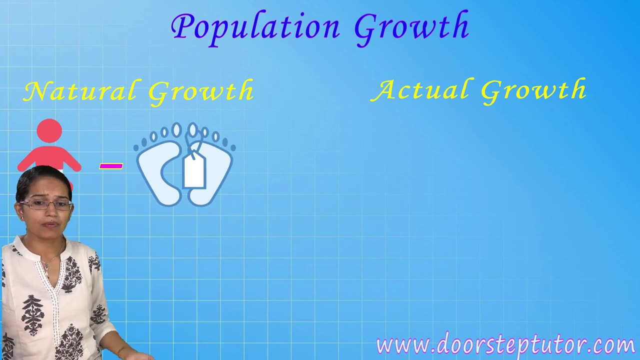 actual population. Natural population is a population which I simply denote by birth rate minus death rate. So, whatever the difference is a natural rise in the population. but when I say actual, there is a very important parameter and that is migration: People who are coming in the 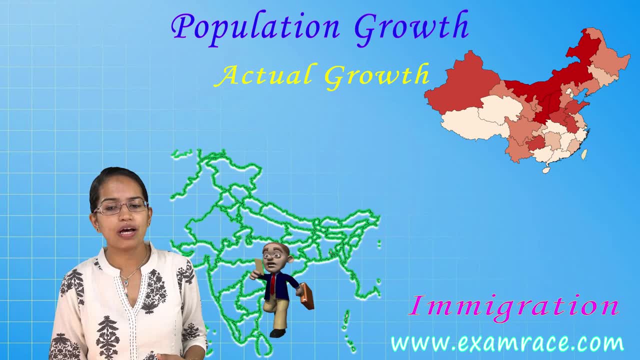 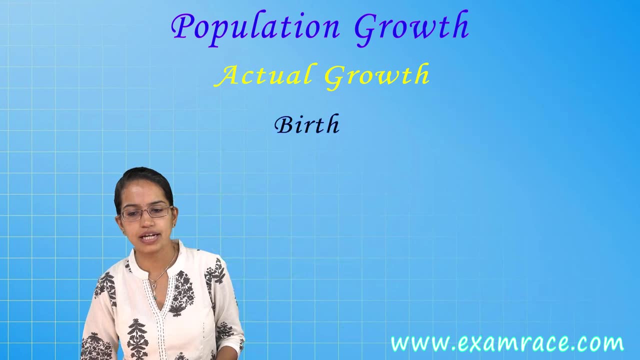 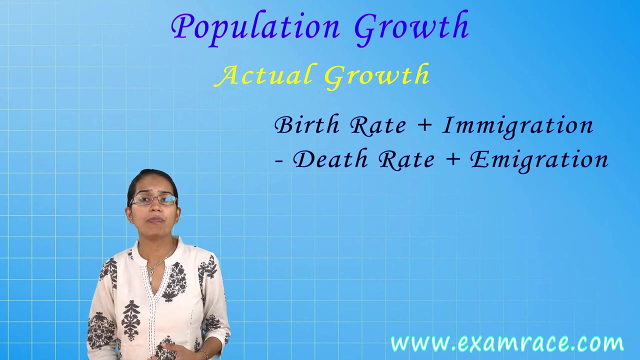 region are known as immigration, So that's in people who are going out, as emigration that is going out. So actual population growth I can say is birth rate plus immigration, minus death rate plus emigration and that's how you have the population growth, the actual population growth. 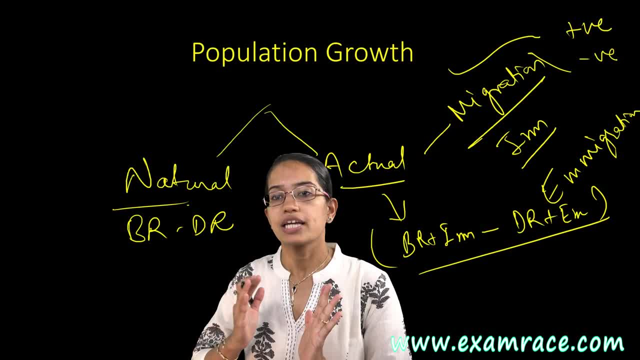 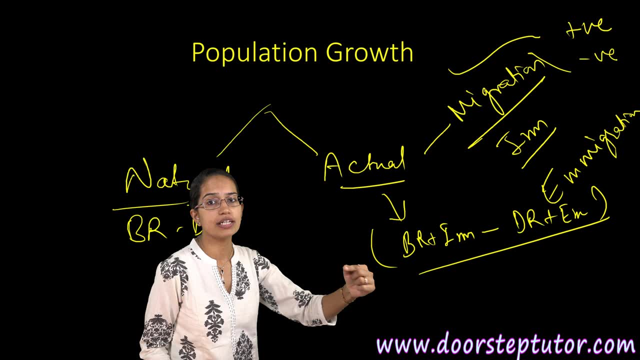 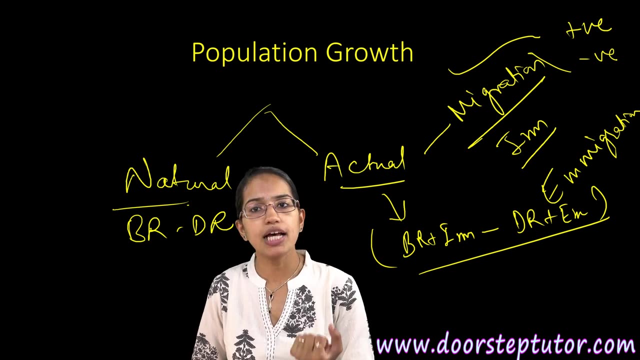 and, as said previously, population growth can be positive, can be negative and when we talk about population change, it's an important indicator to understand the population growth. So, if you understand, the economic development of a region has a huge root, or a well root, we could say, in the 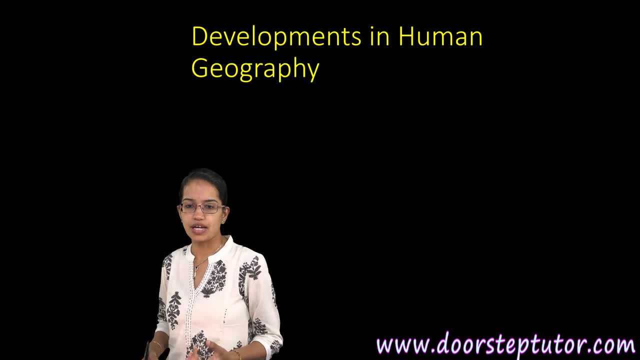 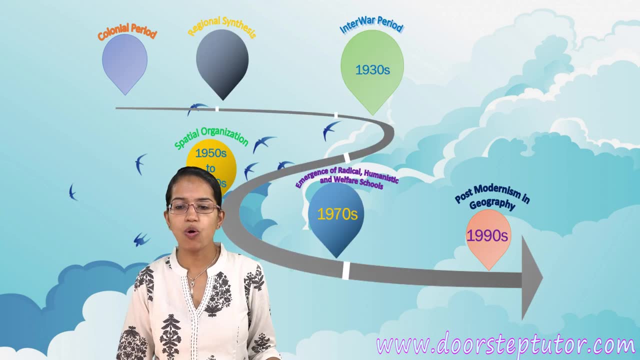 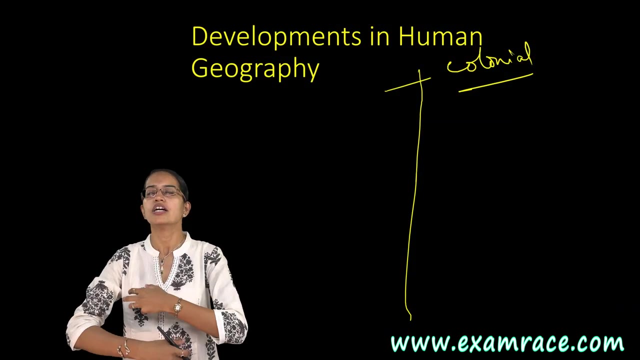 historical and the cultural basis of that region. Now developments in human geography. we have already understood the timeline in the previous class. So with the colonial advent you had the exploration, the discoveries, new lands being discovered, new trade relations being built Later on, during the same colonial period, 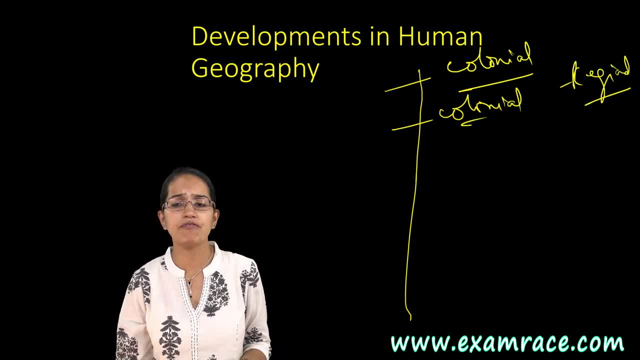 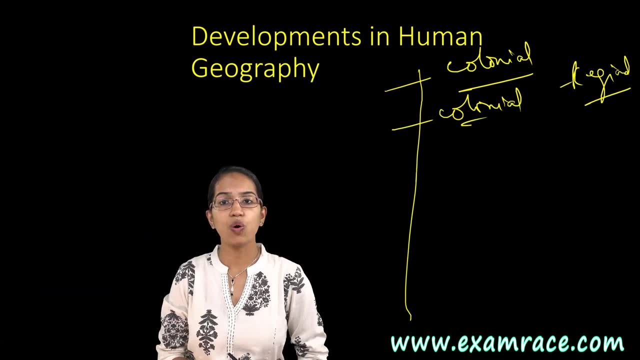 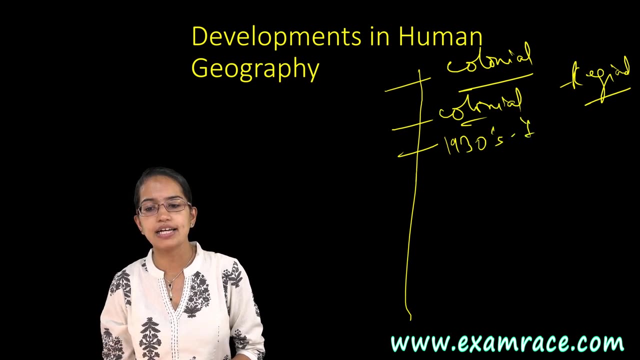 you had the regional synthesis that started, where everyone believed that region to be as one whole. So holistic approach, considering region as a whole, was one of the prior aspects that were discussed. The next important aspect was from 1930s till the interwar period, and this was the time when 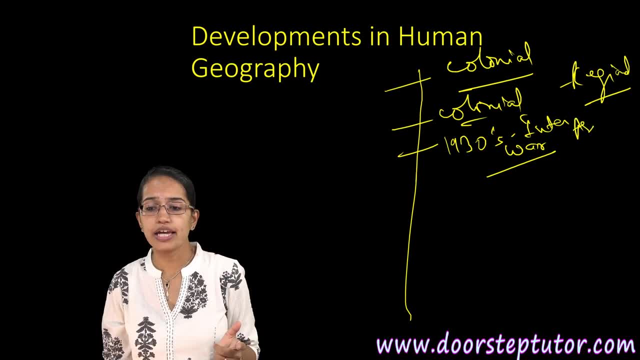 each area was unique to itself, So area differentiation was developed, Be it an area for mining, agriculture, development, etc. So this was the time when each area was unique to itself, So aerial differentiation was developed, Be it an area for mining, agriculture. 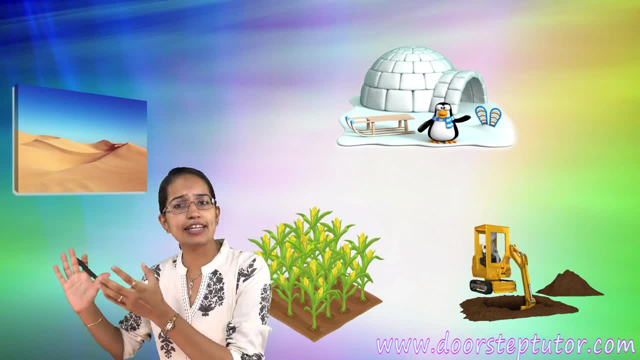 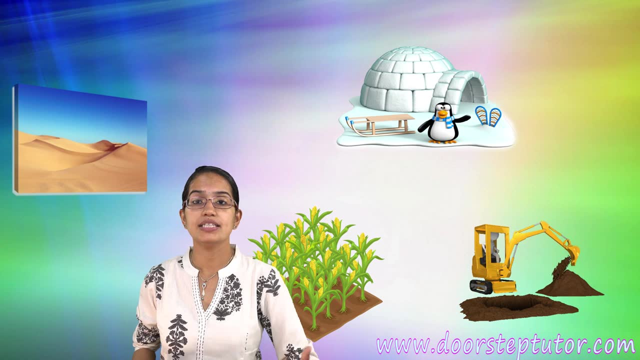 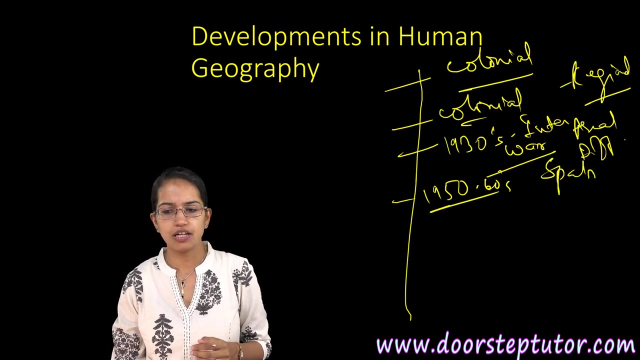 desert, cold areas, polar areas- all had their unique conditions and it was believed that this uniqueness creates the region different from others and this should be preserved. During 1950s and 60s, there was the idea of spatial organization. spatial organization talked about. 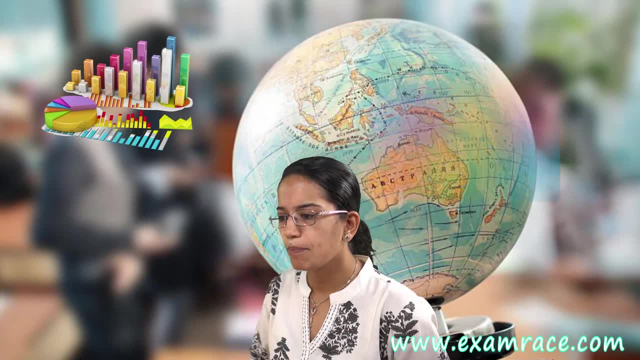 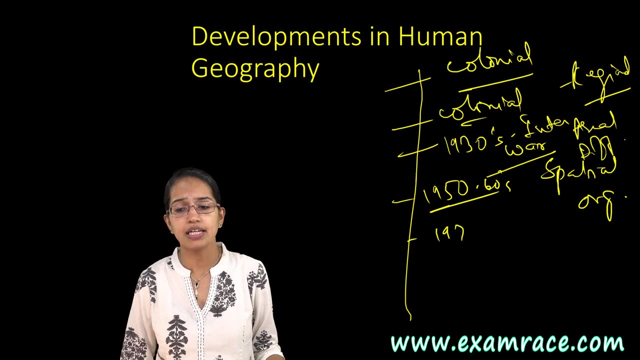 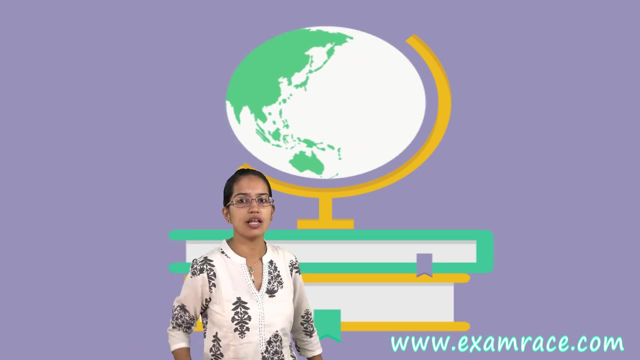 quantitative revolutions. Talking about the statistics, numbers, was some of the basic ideas, but of late it was was realized in 1970s that since geography is a branch of social sciences, we cannot just focus on numbers and quant. We need to understand or relate it to what is in real phenomena. 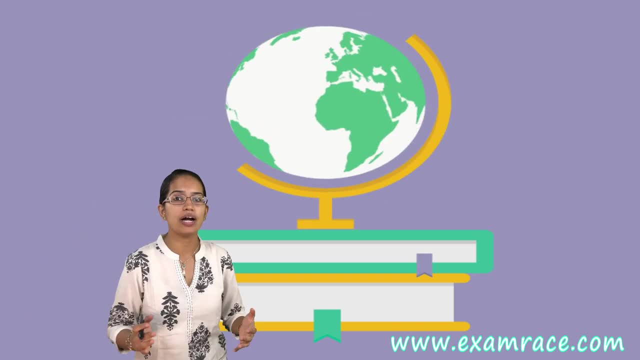 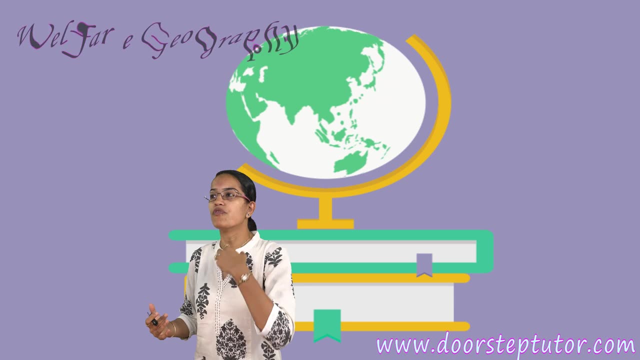 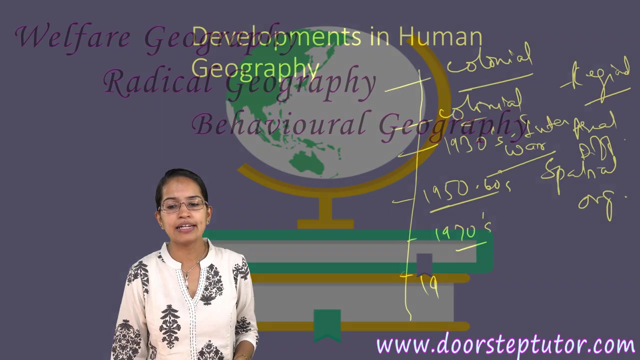 that is, qualitative aspects. We need to understand that there is human behavior which is affecting this dynamics. So welfare geography, radical geography, behavioral geography, started to grow. Later on, in 1990s, we talked about the ideas of post-modernism, which focused on each. 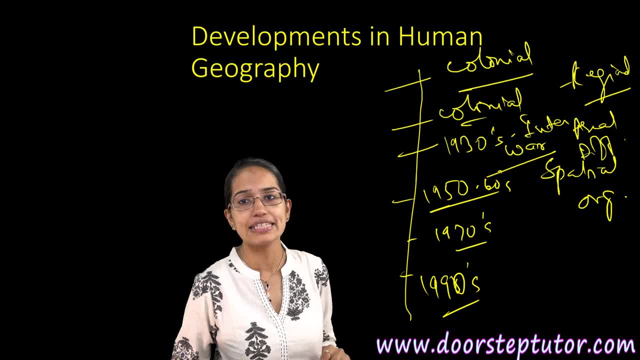 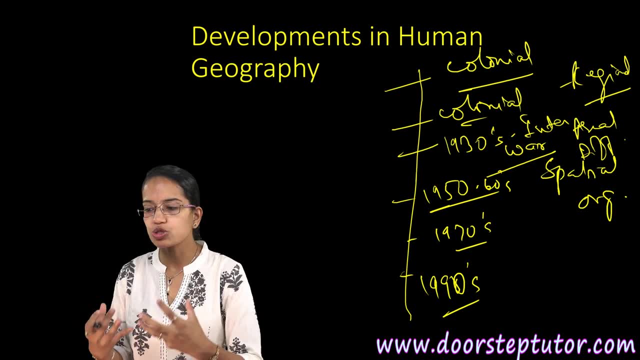 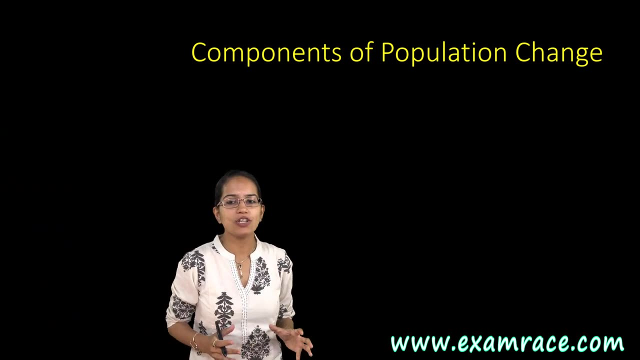 area or each local center being unique in itself, and that unique characteristic would help flourish that area. So emphasis was to explain human conditions or existence of those human beings. Now, as already said, the components of population change are three: Birth, death and migration. 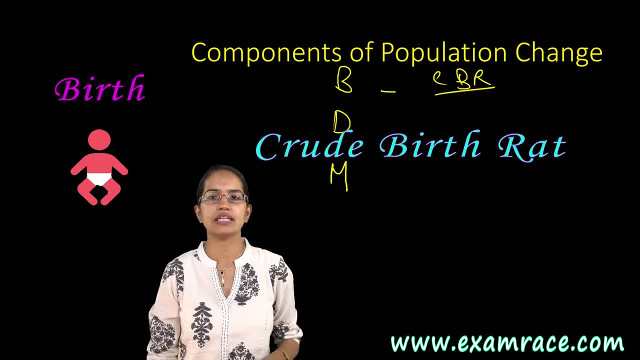 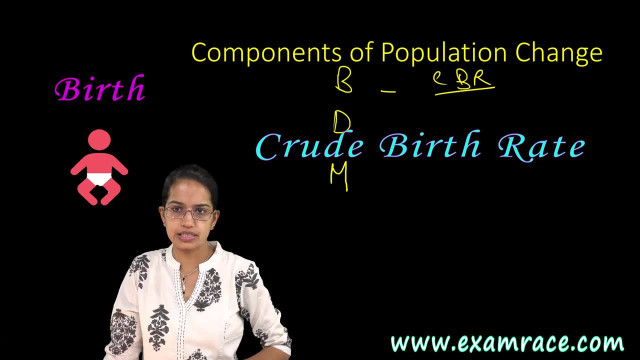 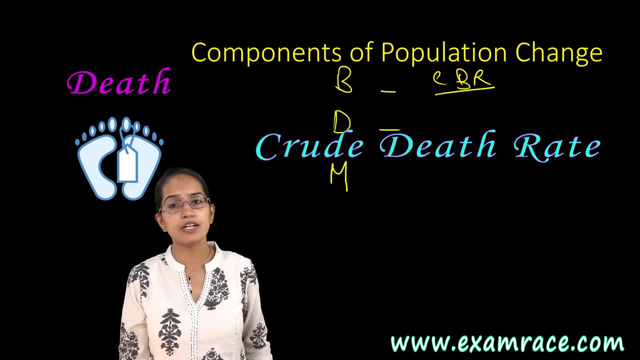 Birth we could explain as crude birth rate. So crude birth rate is actually per thousand women, the number of live births that are there. Crude death rate is per thousand people. the deaths in a particular region is the crude death rate. Migration rate is the number of. 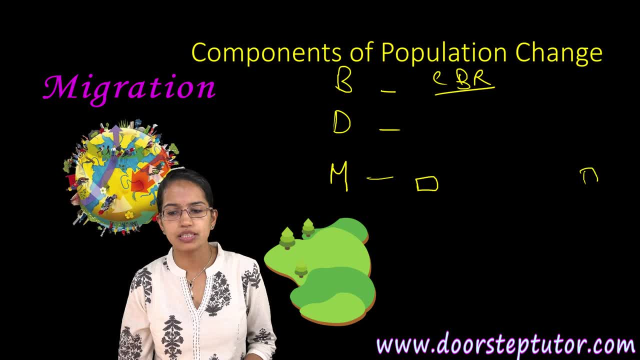 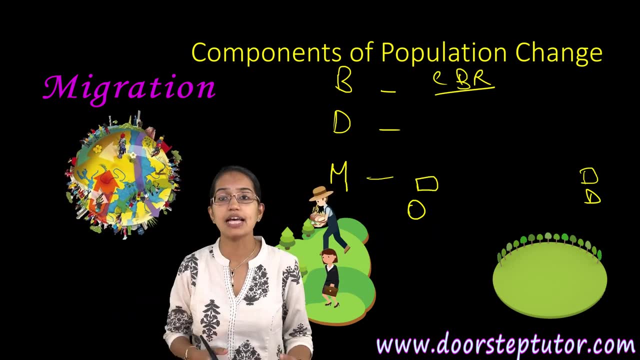 people who die. So the number of deaths in a particular region is the crude death rate. Migration could be understood by a place of origin and place of destination. So there are some people starting to move from a region and they move to the next place and that's. 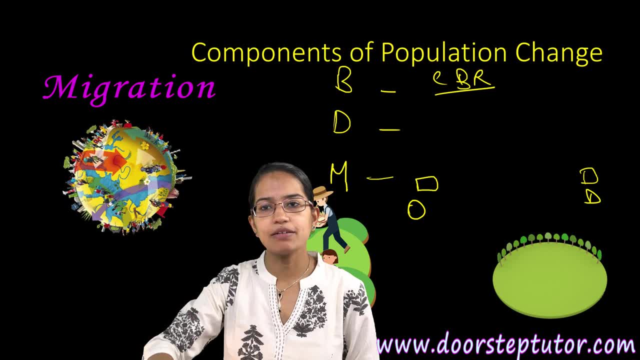 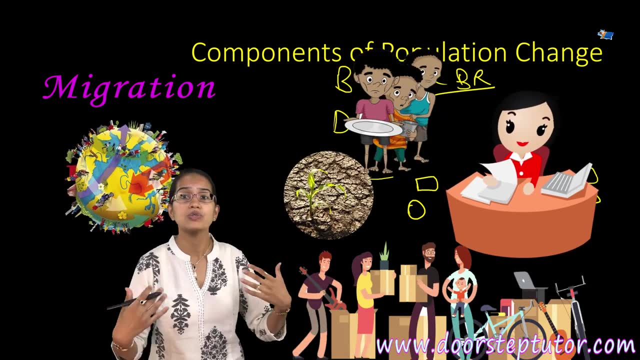 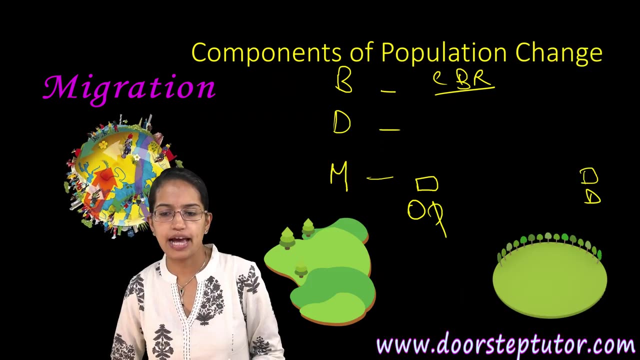 what is migration? Very simple as that. but why they move from this place? This could be due to lack of job, lack of living conditions, famine, drought, disease, war, anything that pushed the people out of this region. So from the origin, I can say there are push factors. 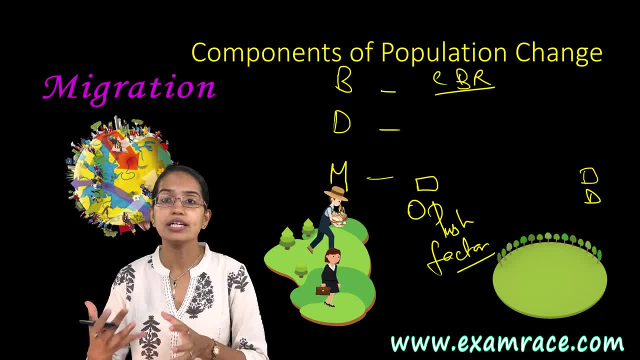 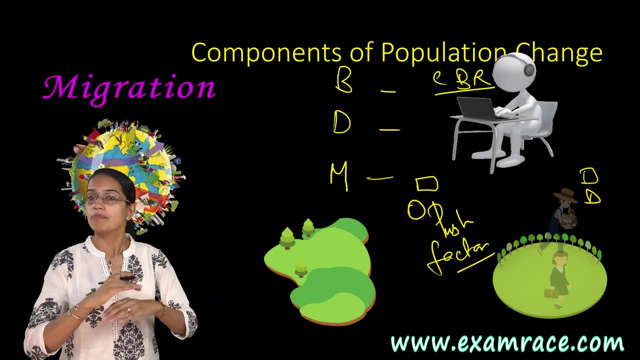 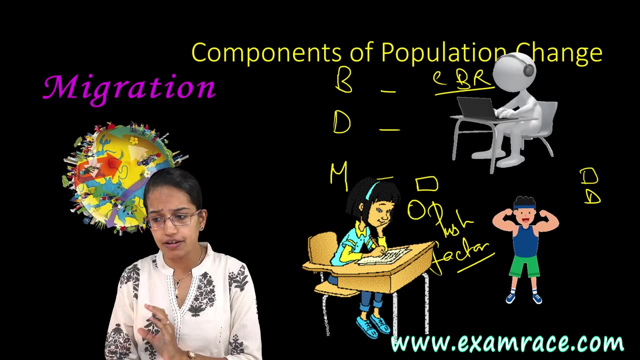 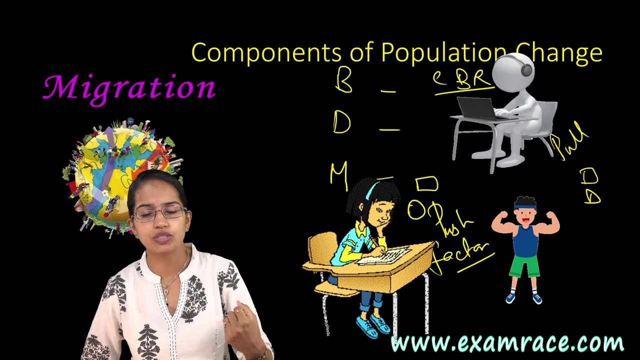 that help people to move out. but, on the other hand, where there is destination, there is always a pull factor. it could be lucrative jobs, it could be better health conditions, good educational opportunities, good lifestyle, a better living condition, more pleasant atmosphere. so what are these? these are the driving forces, driving in forces, and these are known as pull forces. so 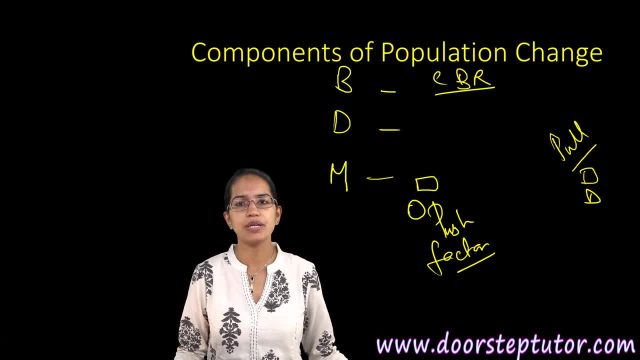 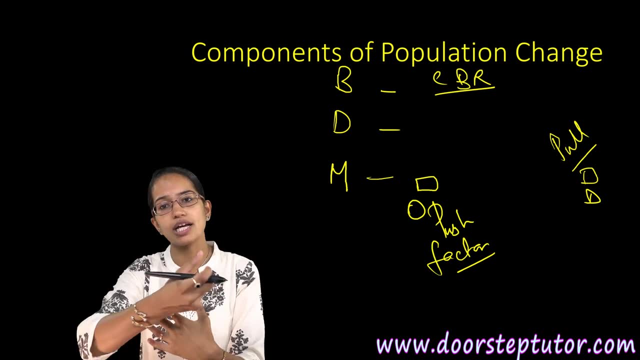 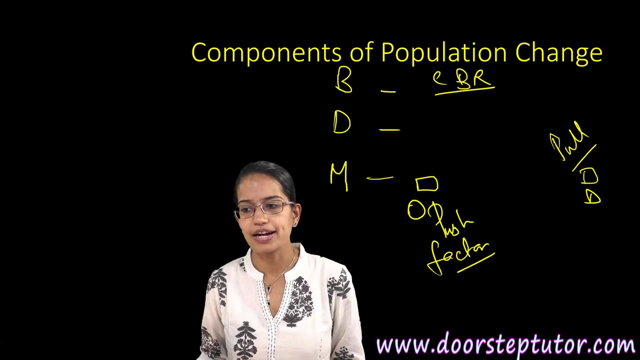 always, when we talk about migration, we understand in the basis of a push factor versus a pull factor. so there are something which is pushing those out, the people out from a region, but on the other hand, some people are attracted towards urban areas- better areas, i would say- and that's a pull factor. 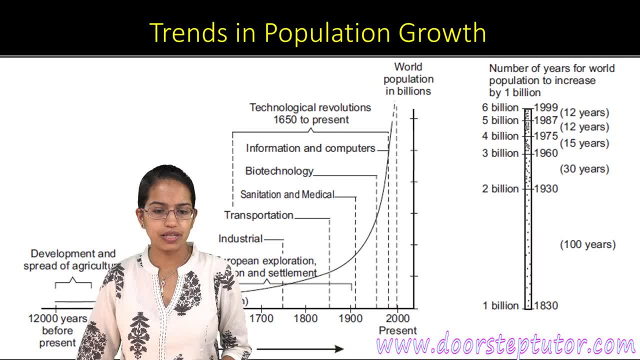 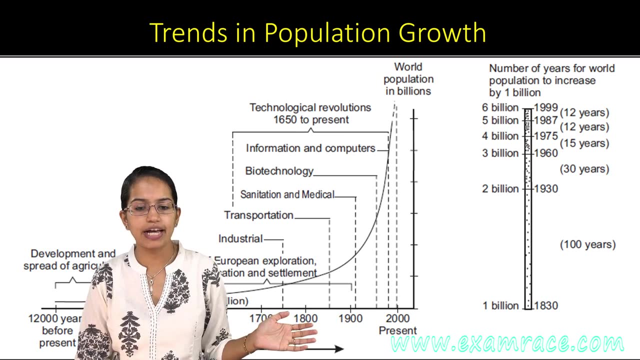 coming on to the next important thing is the trend in the population. so far we have talked about the distribution of the population, the density of the population and the change in the population, but how population grew over years if we look from prior to the birth of christ till 1960s. 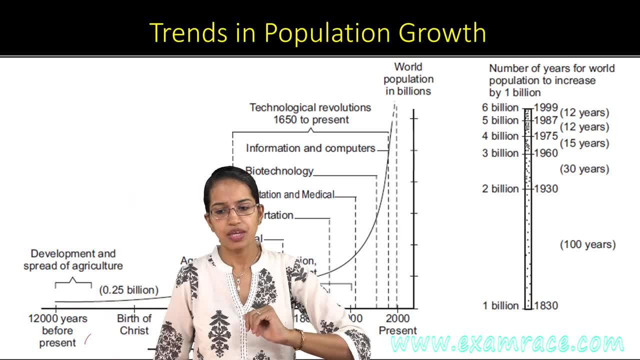 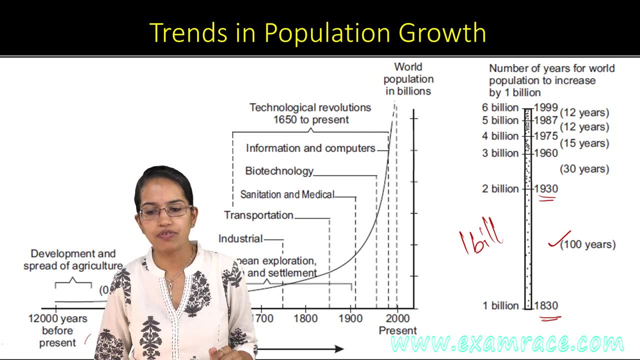 population was only 0.5 billion. from 19 1830s till 1930s, in a period of 100 years, the population grew by 1 billion, but in the last 12 years, if we say, it took only 12 years to have this 1. 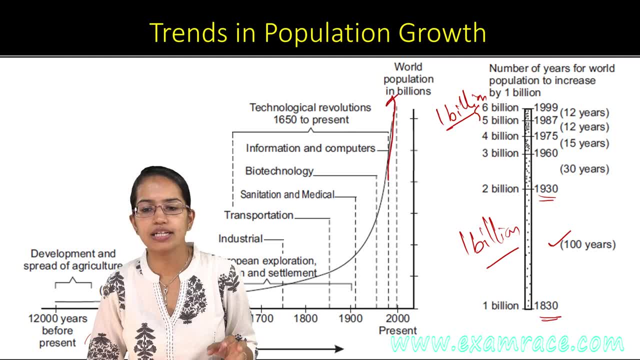 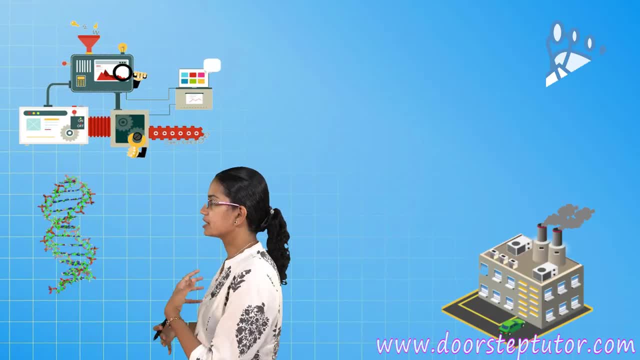 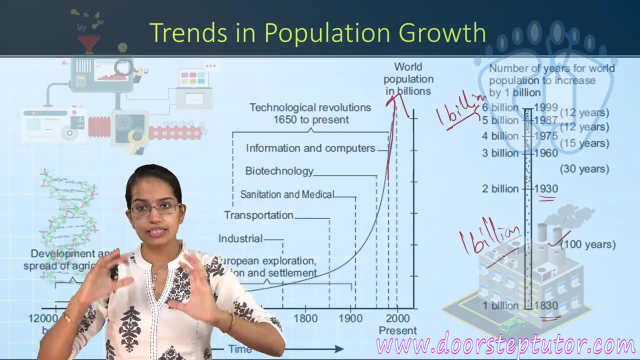 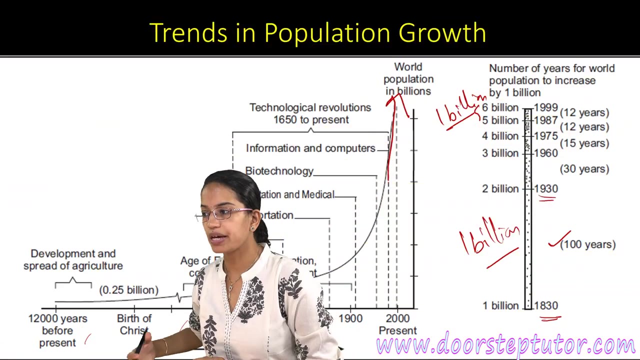 billion population and this is this exponential rise in the population, population that is registered here. so with growth in industries, technology, biotechnology, the death rate was curbed at a very fast pace. the population was basically having a very good standard of living that could be availed to them. the problems of epidemics, diseases, 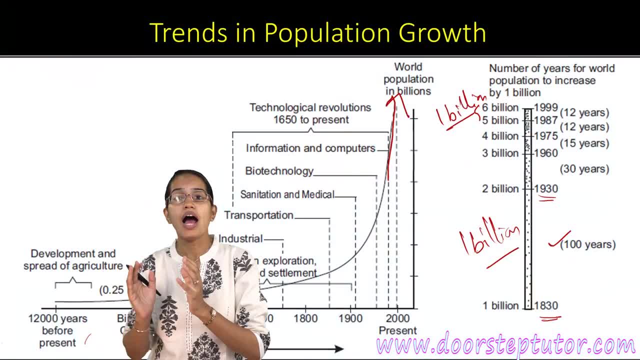 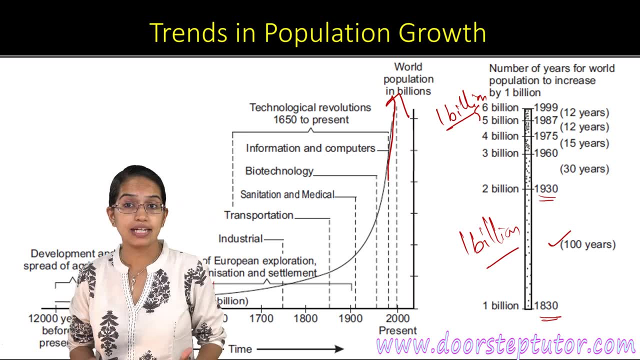 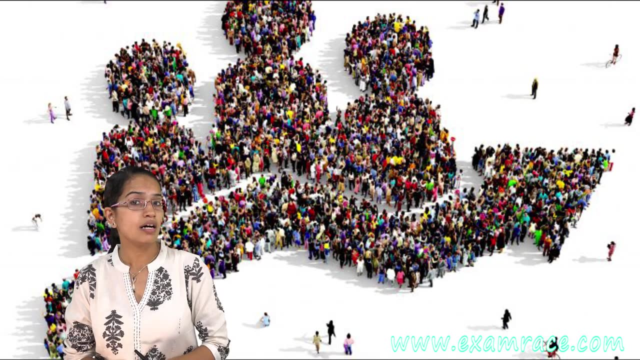 that could be seen were highly curtailed and because of the curtailment of these incidences, there was a sudden decline in the death rate that was registered, and this was one of the major reasons that pushed the population, along with the natural increase in the birth rate. 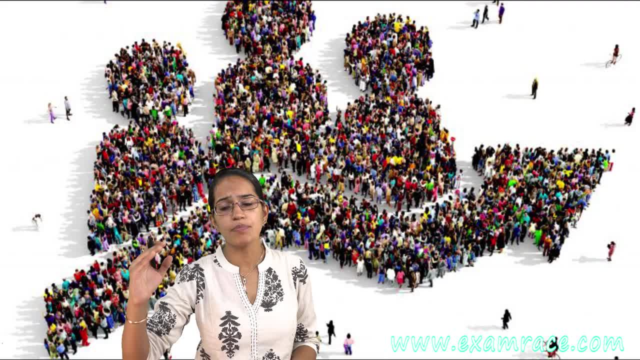 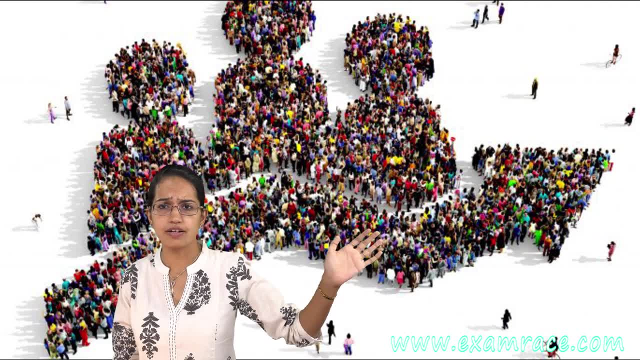 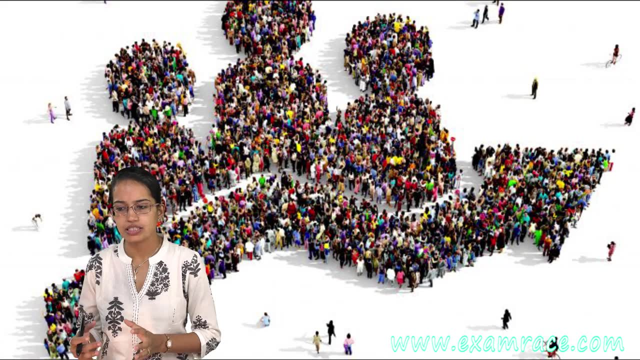 that was seen. so the trend in the population growth has been exponential, we could say from a very less population- nearly 200, 400 years- back to an exponential population in the past 30, 40 years. so this population growth is definitely a cause of concern for the population and 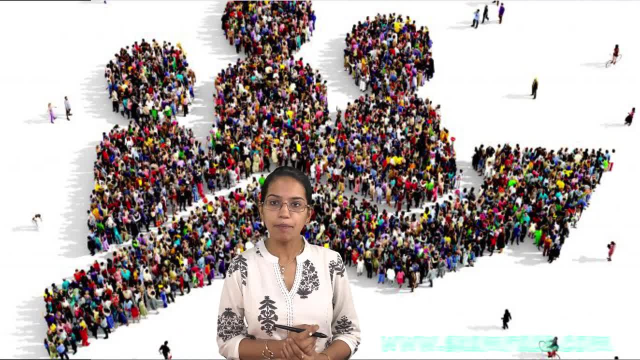 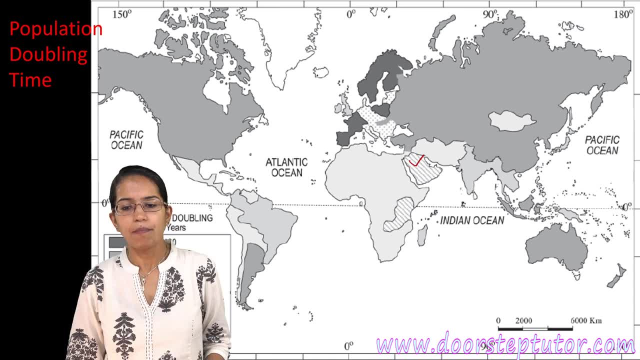 there has been a doubling rate. doubling rate simply says in how much time the population will double in that area. so let's say the regions of Saudi Arabia, parts of Africa. you have a doubling rate of less than 21 years. so less than 21 years the population will. 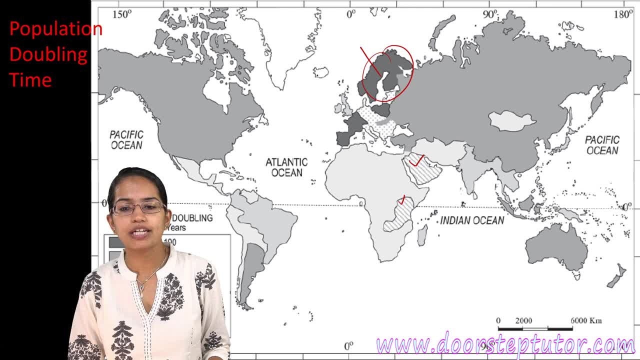 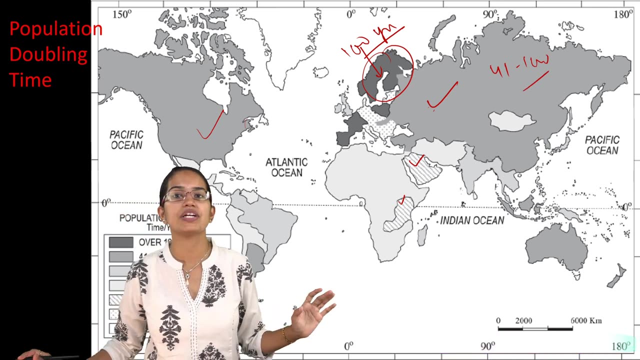 double. but in the parts of Europe here you would take more than 100 years to double the population. however, in parts of Russia, America, parts of Eastern Europe, you have population of less than 200 years to double. So different areas across the globe have different doubling time. on the other hand, there are parts 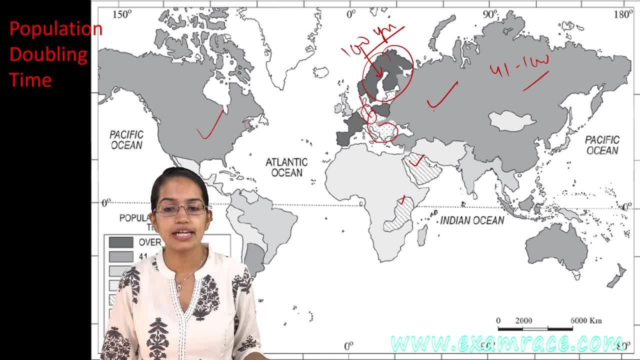 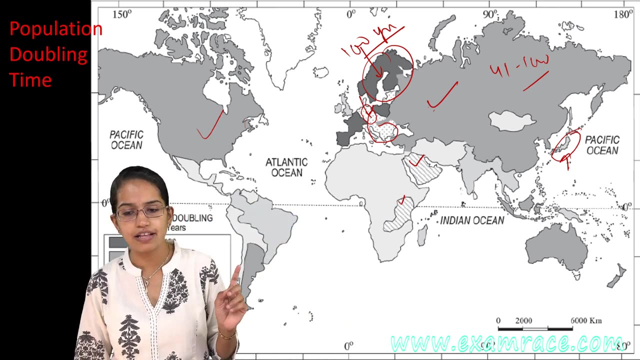 of France, Germany, where you have registered a negative growth rate, a declining population, and similar. now is the case with Japan. that has been talked about, where we talked about declining population. Now, one more important thing to understand here is in India, we say the annual average population growth rate is 1.9 percent. that means within every thirty six years, the age 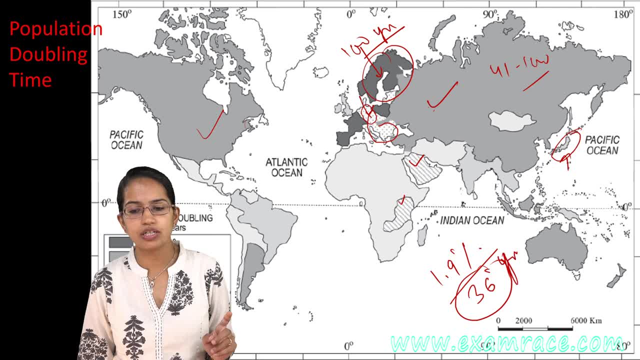 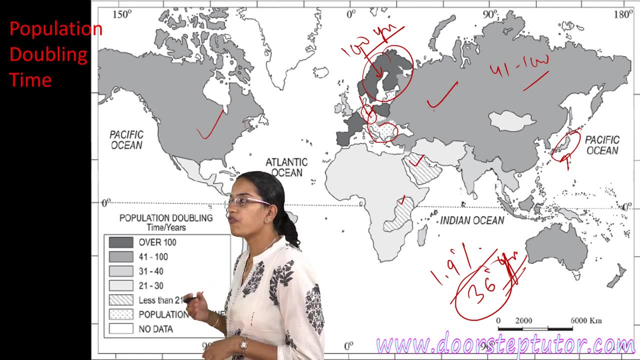 of growth to be reached. that is the annual average population growth rate. in India it is 1.90 percent. population would double up. However, for other developed nations it takes more than 318 years to double the population. So for us it is a very big challenge to curtail the growing population. 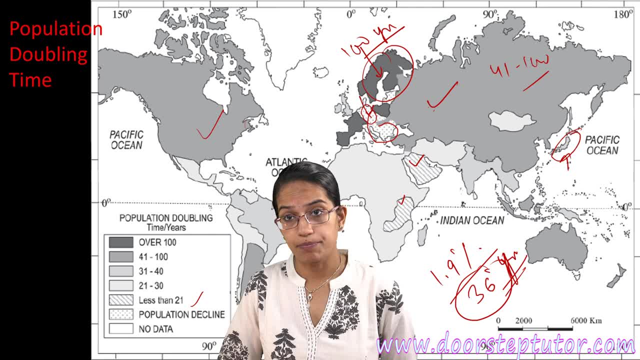 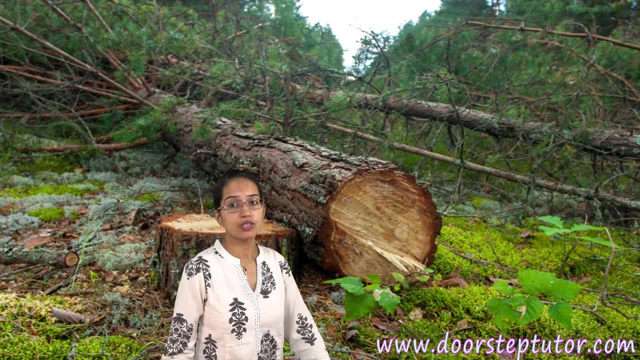 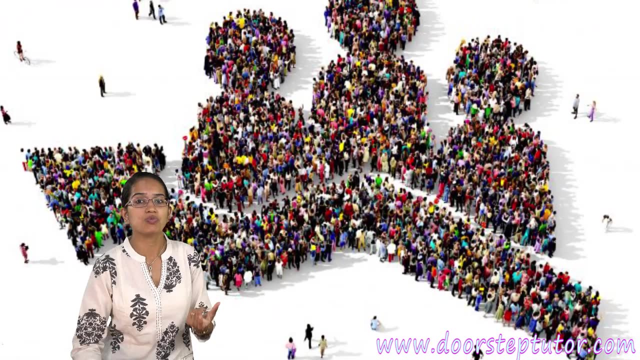 Now this dynamics has led to severe implications. Now implications are in the form of depletion of the resources. Whatever resources we have would be exhausted at a point. So if you have a constantly, ever rising population, it won't be able to sustain, And Malthus was one to point this out. 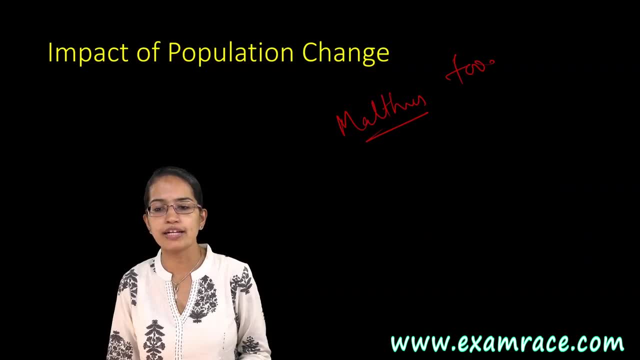 So Malthus, under his theory, predicted that there is food and population and the relation of the food is arithmetic. So the food resources grow 1,, 2,, 3, 4, but the population grows 1,, 2,, 4,, 8.. 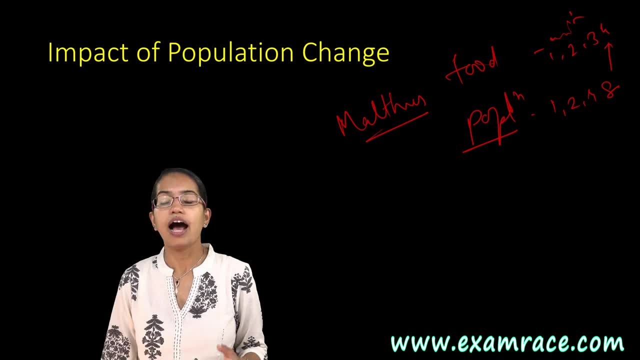 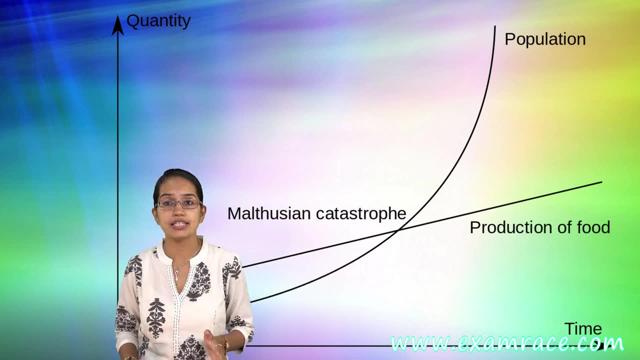 So this 4 has to match this 8 and that's a huge gap. So the idea is, at a point there would be a sudden crash where you would realize that this food is not able to sustain this much population. And that's how we understand that if the population grows on. 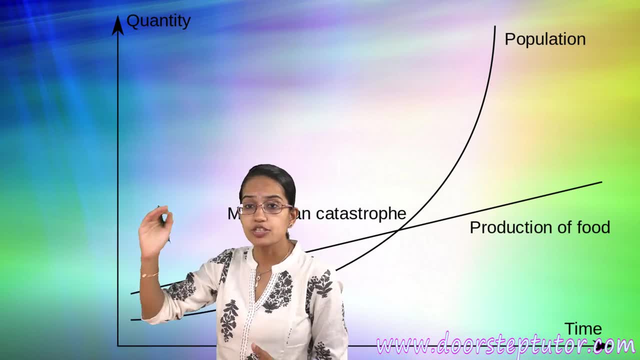 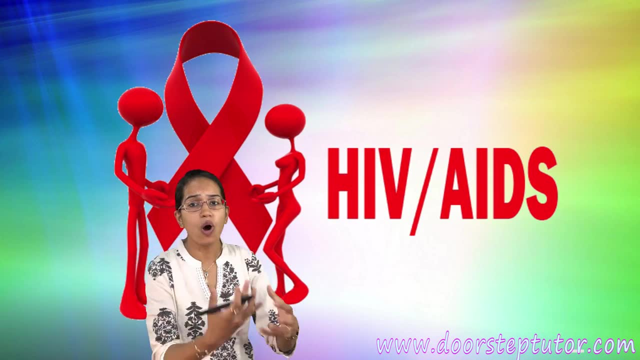 continuously, there would be a point where there would be a saturation level that would be reached. You have numerous epidemics that are being talked about- HIV, AIDS. All these lead to lower life expectancies, higher death rates that have been registered. Again, you have the demographic. 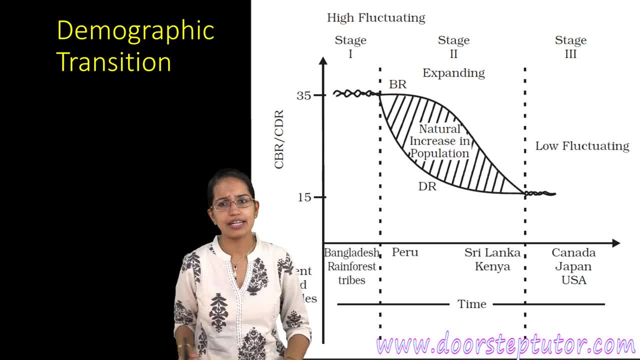 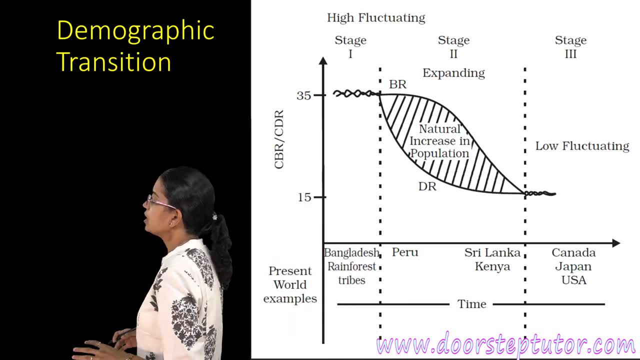 transition theory. You have usually four categories, but NCRT has given three here, So we'll discuss it in the next video. So thank you for watching Now. the idea is, under this demographic transition we have a transition from a rural, agrarian illiterate. 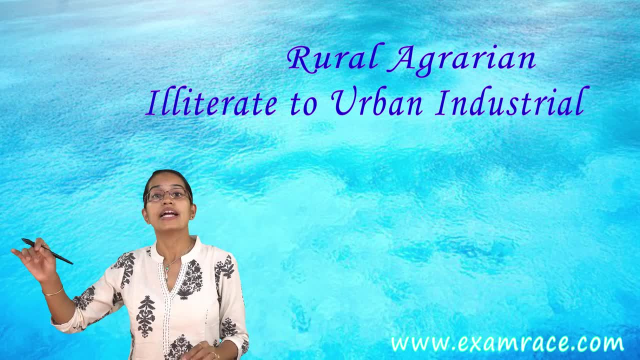 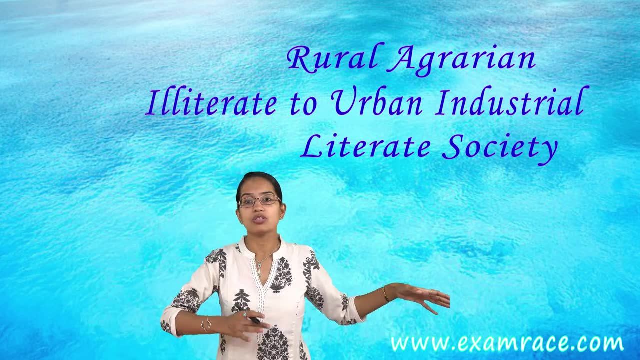 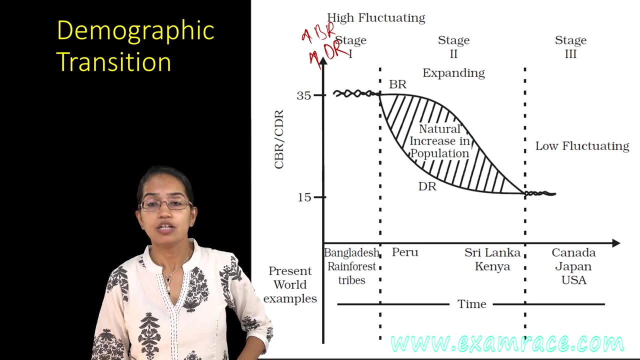 society to an urban, industrialized, literate society. So that's where we want to move, from where we were Now. this happened in three different stages. The first stage was a stage of very high birth rate and very high death rate. So people birth taking place in a very high birth rate. 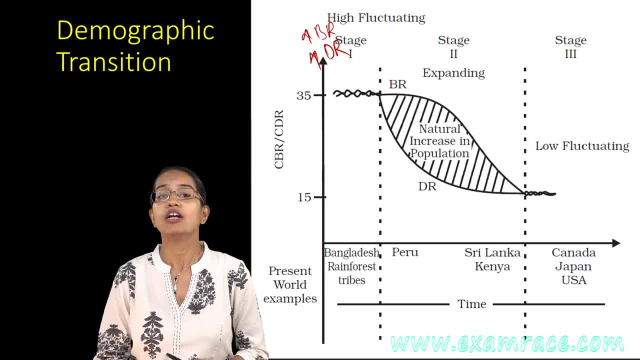 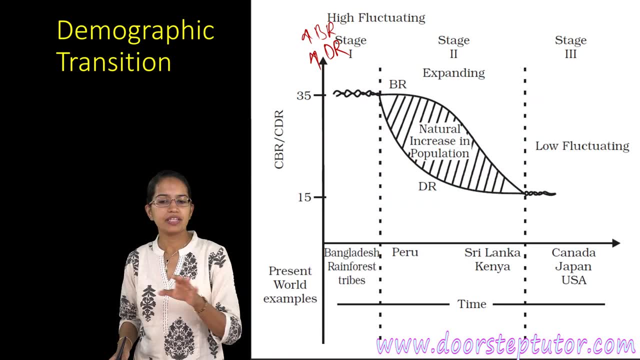 at a very high rate and death also at a very high rate. Lot of epidemics, lots of diseases. So there was no growth in the population, Absolutely no growth in the population, and everything was stable. Presently seen in the parts of Bangladesh rainforest tribal areas. The next stage was a 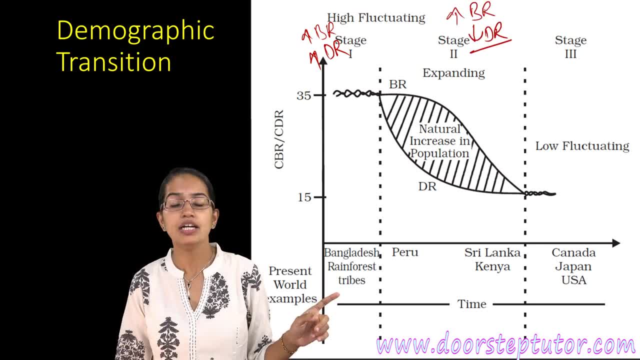 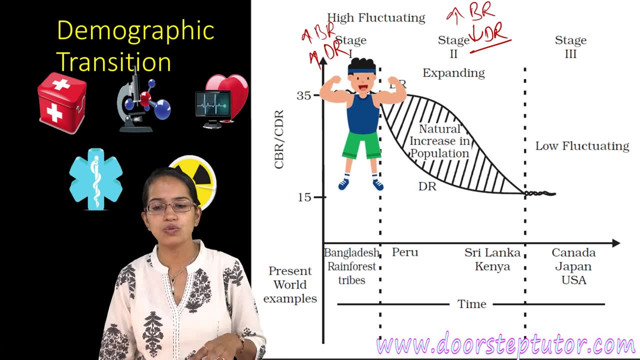 stage where birth rate was high but death rate was curtailed due to better medical facilities, good health conditions, control of epidemics, control of diseases, But this led to a very high or natural increase in the number of deaths. So this is a very high rate. So this is a very high rate. 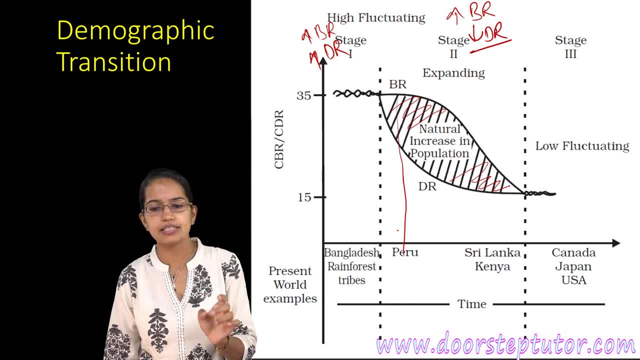 Regresing population. The earlier part of this expanding series has been witnessed in Peru, and the declining phases are seen in the regions of Sri Lanka and Kenya. However, the last stage talks about a declining birth rate, along with a declining death rate. Now how did the birth rate decline here? 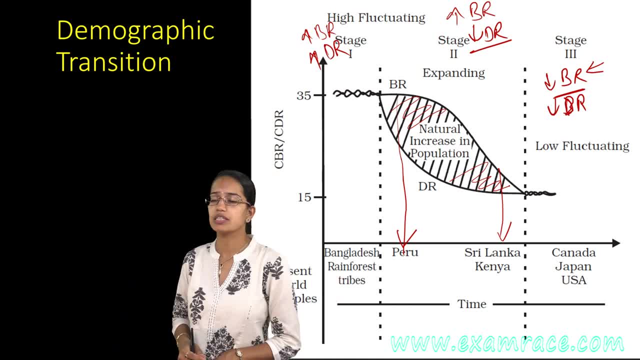 The birth rate. the major factors that affected the decline of the birth rate were more awareness, postponement of the age of marriage, better family planning that was adopted and, ultimately, more awareness in living conditions. So many of these things were happening during this period. So the 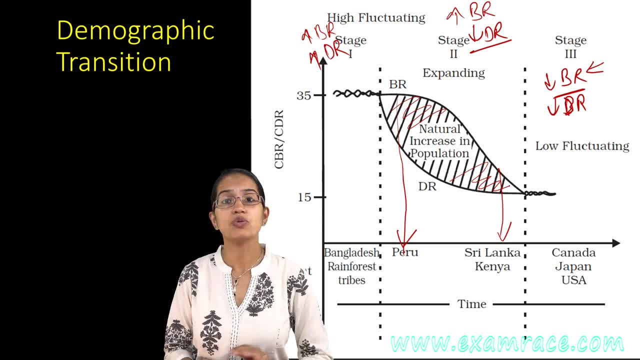 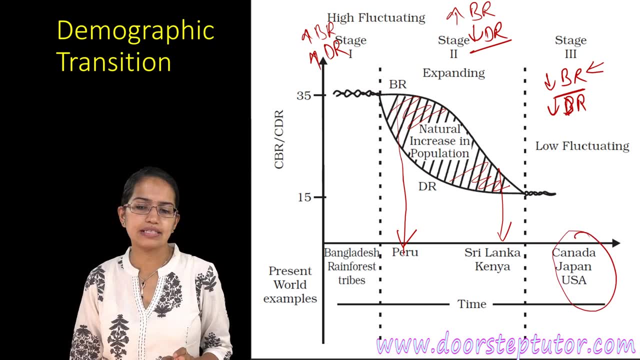 propaganda, tax disincentives given to bigger families were some of the reasons that led to decline in the population, and this was mainly seen in the regions of Canada, Japan and US. So here again, you would have a decline in the population that was registered. 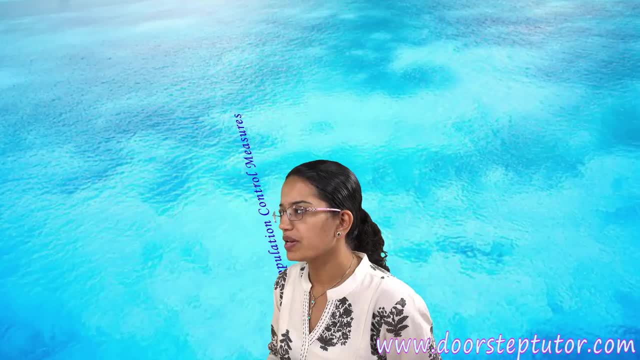 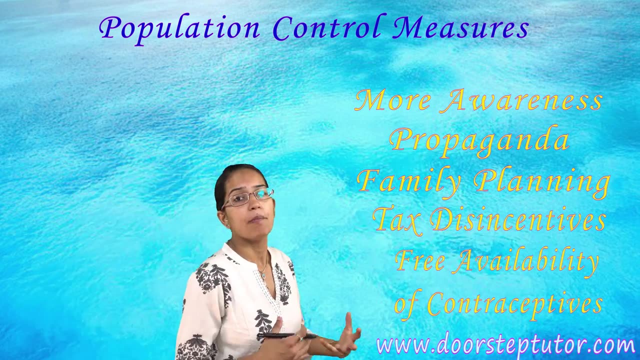 The next important thing we need to understand is the population control measures. So awareness, propaganda, family planning, tax disincentives are some of the major ways- Malta's aspects that we have already discussed- where we have the preventive and the physical checks that are important. 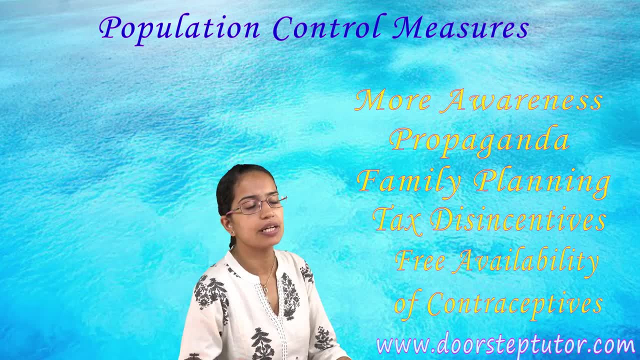 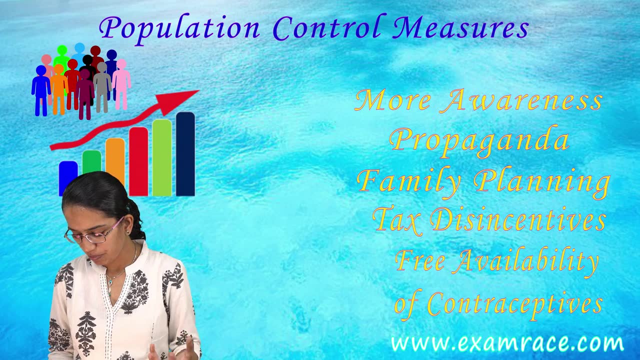 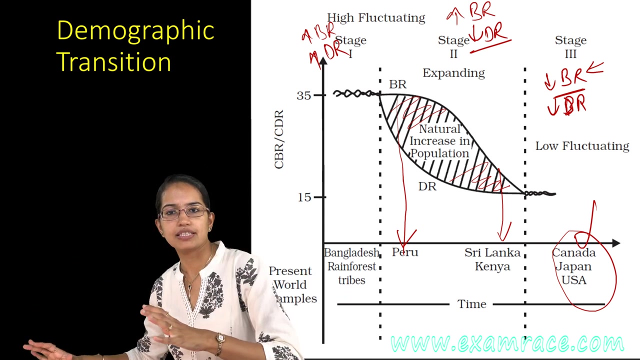 to curtail the growing population and for sustainability of our resources. definitely, this ever-increasing population must be checked, and only when this ever-increasing population is checked you could have a better lifestyle, a better, healthier life. that could be seen. So this demographic transition model is all about describing and predicting the future. 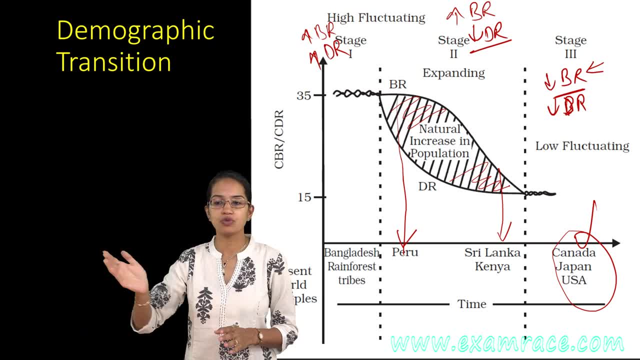 So what we have at present is this: what would be the future could be predicted from the demographic transition model. So what we have at present is this: what would be the future from this demographic transition model, A very important part in your human geography section? 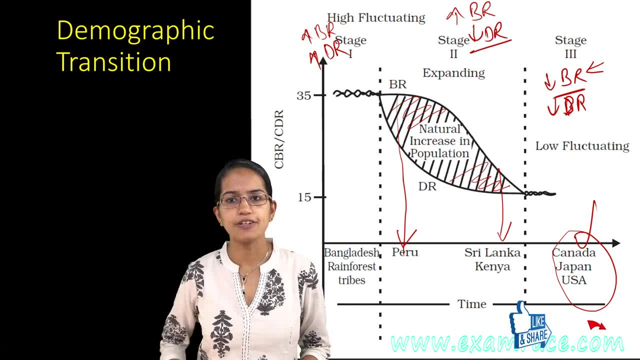 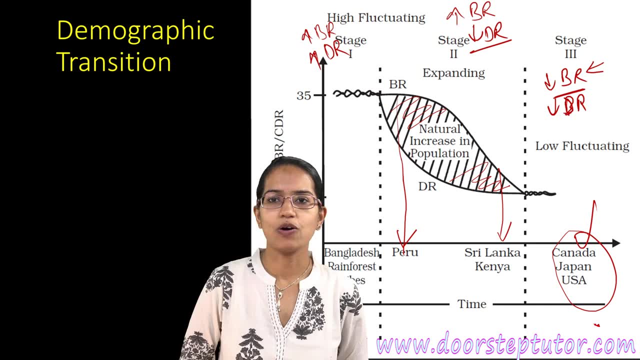 demography, population studies. We'll be doing a lot many topics under this section, So keep subscribed. Have a wonderful day. For any doubts, leave those in the comment. I'll be happy to resolve those personally. Have a wonderful day ahead. 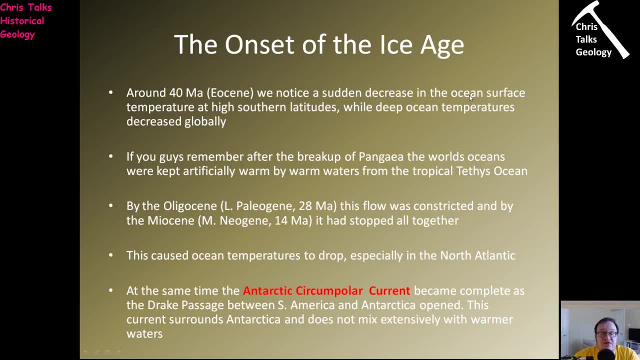 Hello everybody and welcome to the next part of Cenozoic Earth History. So, as you can see from this slide, we're going to be talking about the onset of the Ice Age. Now I should point out that when we're talking about the onset of the Ice Age as part of this presentation, we're doing it in a